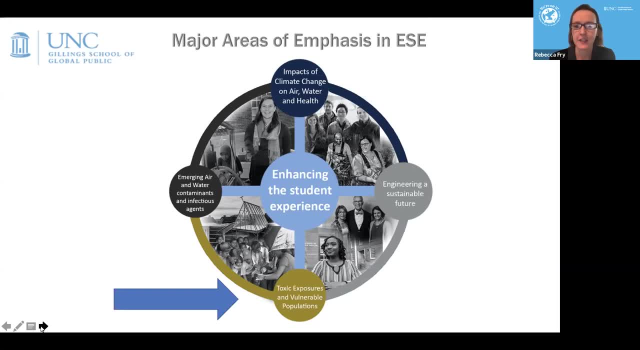 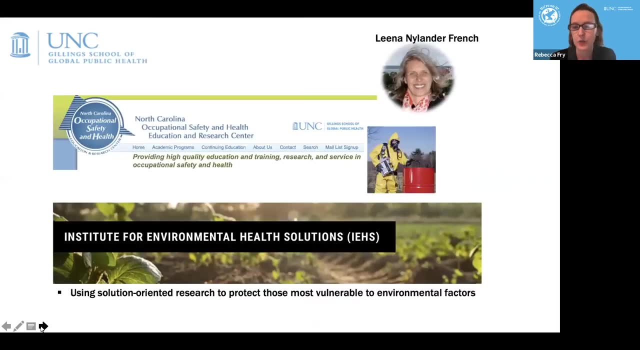 engineering assistance and sustainable future, And then, related to what Dr Sook is going to talk about today: toxic exposures and vulnerable populations. Two of the entities that we house within the department that focus on vulnerable populations and their protection is the North Carolina Occupational Safety and Health Education Research Center that's led by Dr Lina Nylander-French, focusing on occupational safety and health. 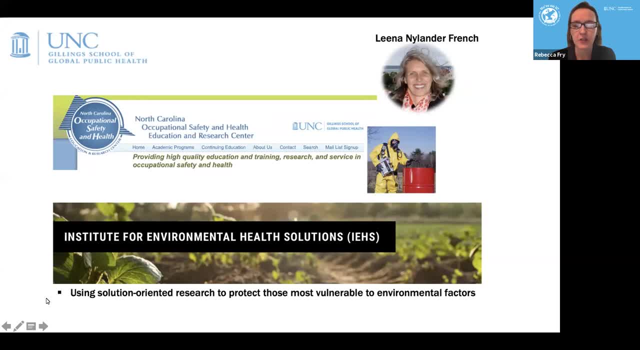 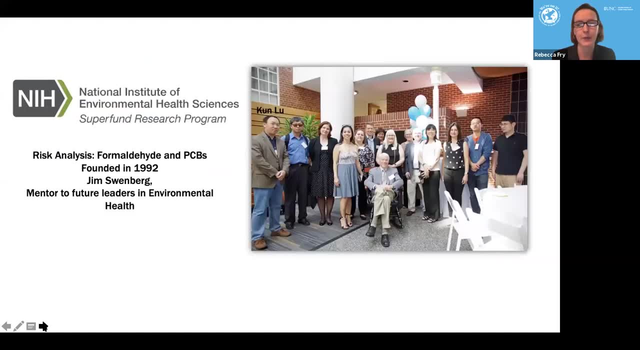 of different populations And also the Institute for Environmental Health Solutions, which I run, where we use solution-oriented research to protect our vulnerable populations. Our department's also very familiar with the NIEHS Superfund Research Program. Our first Superfund Center was founded in 1992 by Dr Jim Swenberg. It had a focus on risk analysis and researchers' 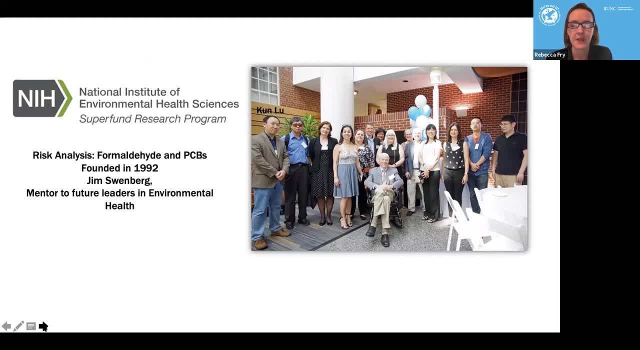 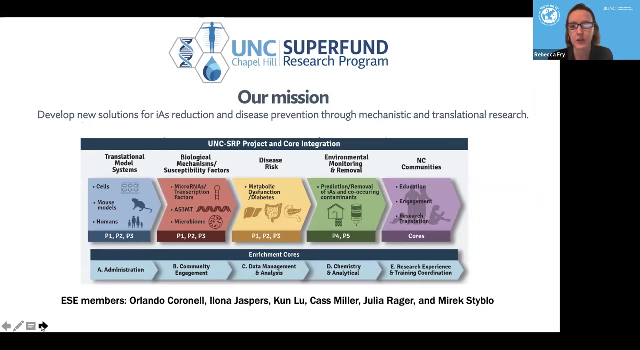 focus their research on formaldehyde and PCBs. Here Jim is pictured at his retirement ceremony, surrounded by his mentees, many of whom have gone on to be leaders in environmental health. One example is Dr Kun Liu and our department, who's an expert in exposomics in the microbiome, and I'm so honored to be the director of our newly funded Superfund Research Program. Our contaminant of focus is inorganic. 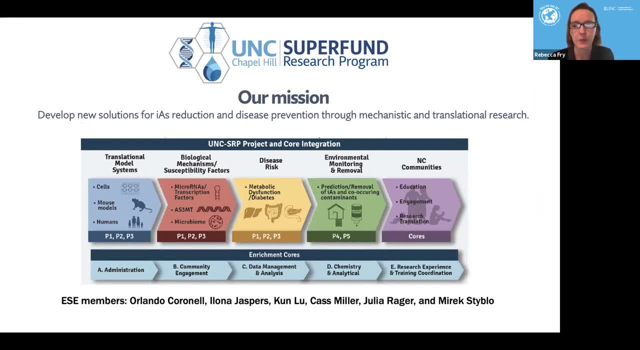 bacteria, inorganic arsenic and through interdisciplinary research, we're working on reduction and prevention of disease through both mechanistic and translational research. I am honored to be surrounded by amazing scientists, including ESE members, Orlando Cornell, Ilona Jaspers. 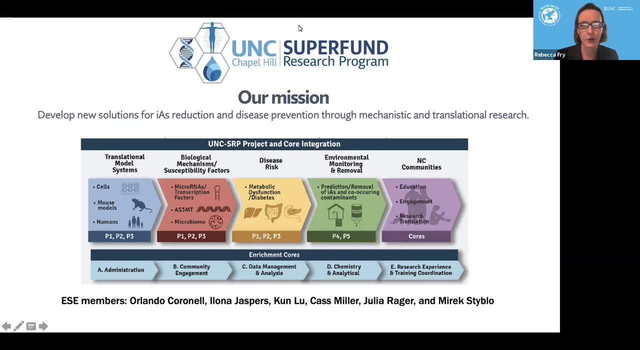 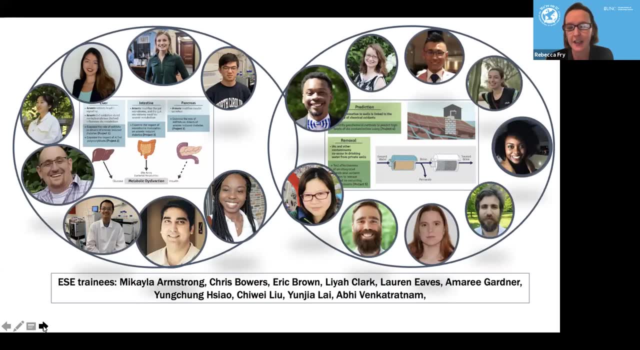 Kun, Liu Casey Miller, Julia Rager and Marek Stieblo, who are all contributing to this team focused on risk reduction of inorganic arsenic. And one of the wonderful components of the Superfund Research Program is its support of trainees, and I've highlighted some of our 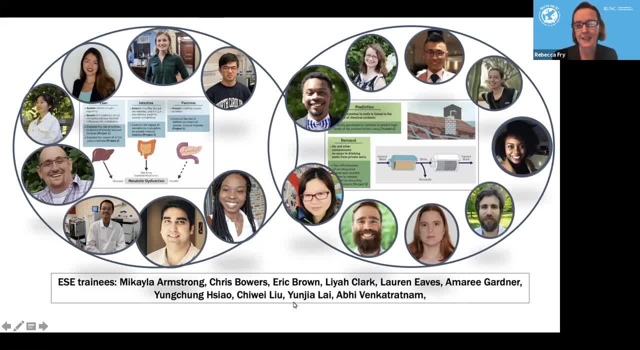 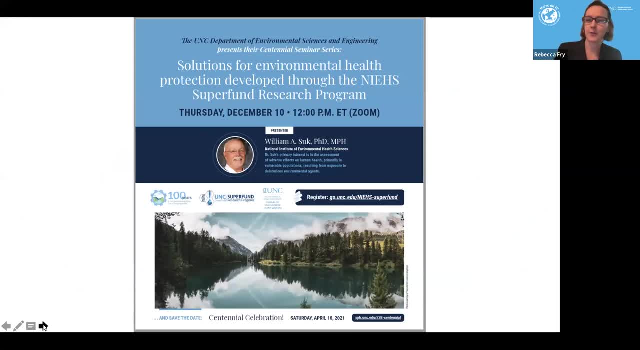 trainees here, listing our ESE students here at the bottom. So we're so looking forward to Dr Suk's seminar and his perspective on solution-oriented research that's coming out of the NIE. Dr Suk received his Bachelor's of Science and Master of Science in Biology from American. 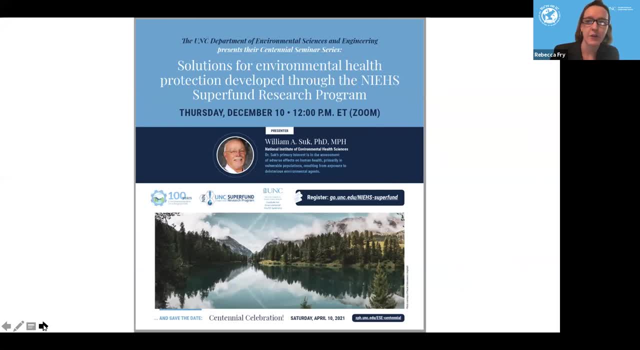 University a PhD in Microbiology from George Washington University, and he's alum of the UNC School of Public Health, with a Master's in Public Health Policy and Management. His primary interest has been the assessment of adverse effects on human health, particularly vulnerable populations. He has a long career focused on research and research and he's been a 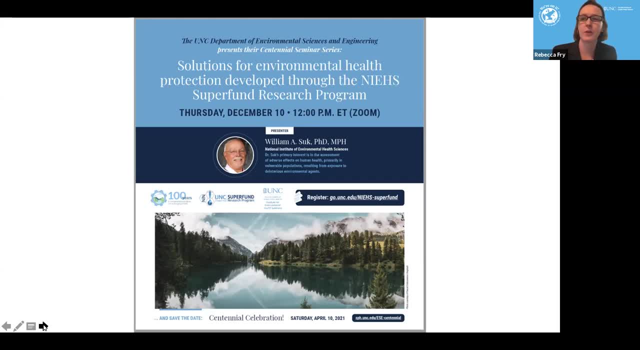 director of the Center for Environmental Health Research on Protecting Children Around the World from the Harms of Environmental Factors. He's the recipient of so many awards that I won't have time to read them all, but let me tell you about some of them: The NIH Award of Merit. the DHHS. 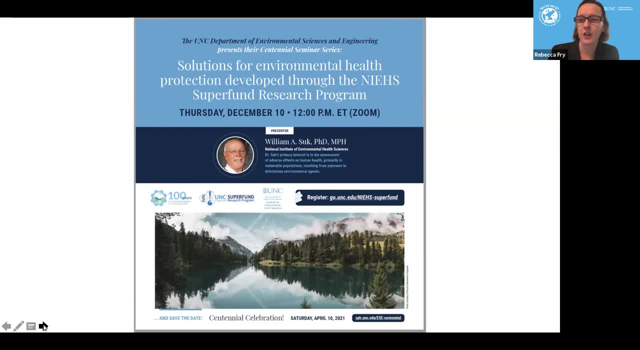 Secretary's Award for Distinguished Service Child Health Advocacy Award from the Children's Environmental Health Network, the Society of Toxicology Founders Award. He's also a fellow of the Collegium Ramazzini. He's also a member of the College of Environmental Health and 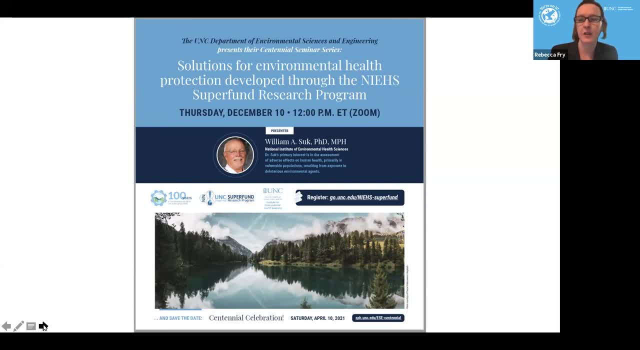 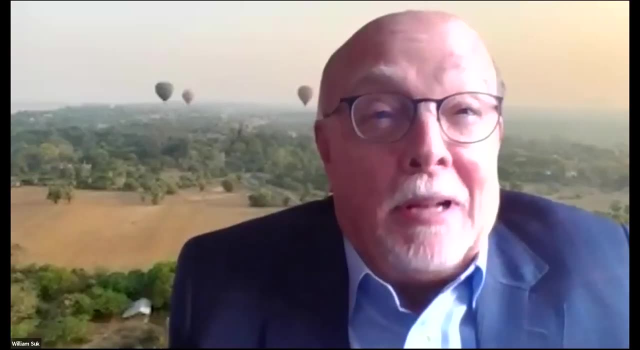 the International Society of Scholars in Environment and Occupational Health. So, without further ado, let me welcome Dr Bill Suk. Thank you, Bill, for being here today. My pleasure, And you said it all. I mean, I don't really have to even go any further, You've. 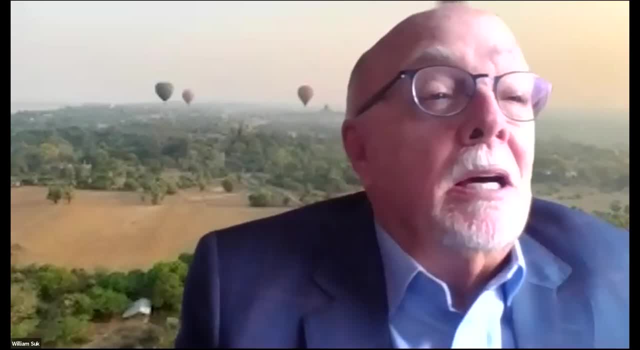 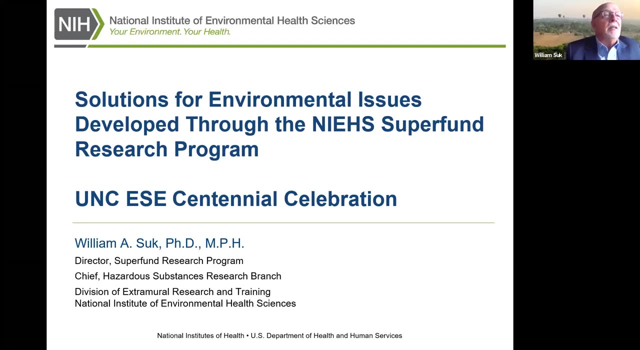 done the whole job right there. I'm going to ask Rhoda to put my slides up, please. We've had a somewhat of a glitch in my presentation, so you're going to hear me say next. So first of all, I want to thank everybody at UNC for inviting me. 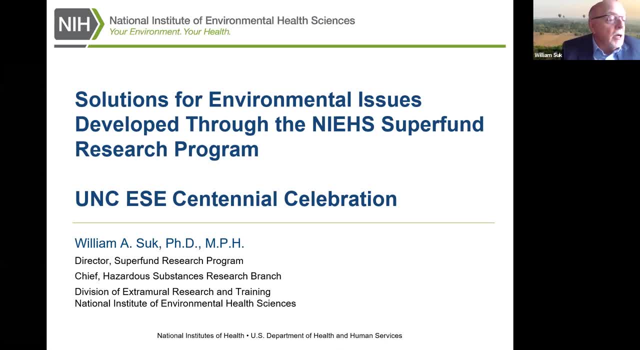 providing an overview of the program and to be able to give you some thoughts about where I think we might be going. Next slide, please. So this is what I'm going to talk about. I'm going to provide an overview. We're going to talk about what we're going to talk about. We're going to talk about what we're. 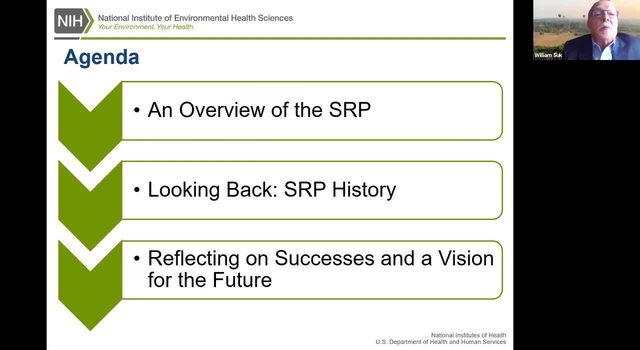 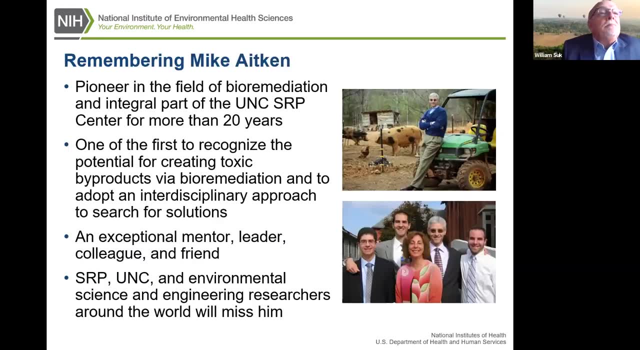 going to talk about. We're going to talk about what we're going to talk about. We're going to look back a little bit in history and we're going to reflect on some of the successes and a vision for the future. Next, please. However, first, I wanted to tell you: 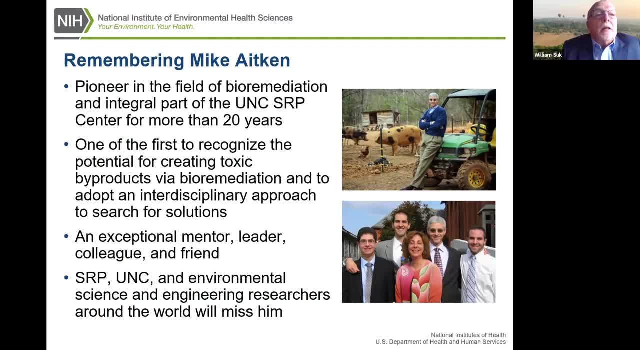 that I want to start off by remembering Mike Aiken. You know I'm not going to go into a lot of detail. You know more about what Mike has done than anybody else, But I do want to say that, um, he was, or was, an exceptional mentor and a leader, And he was also a very good friend. 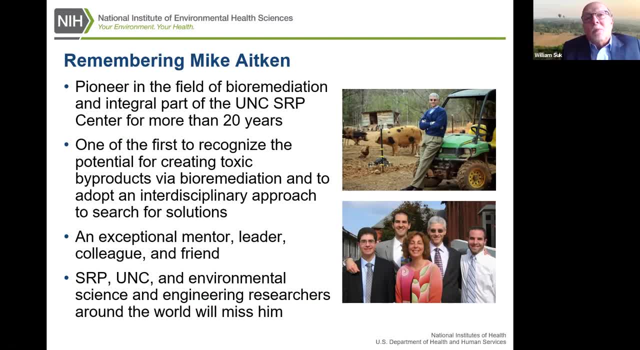 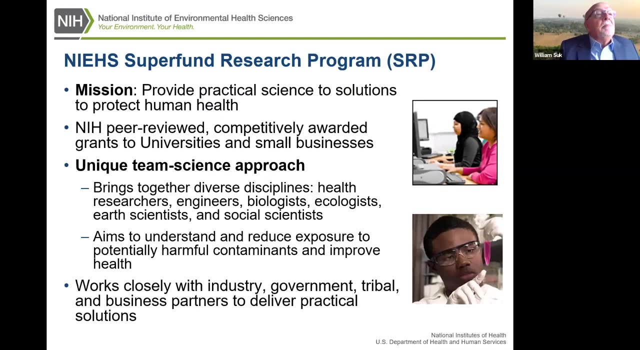 and colleague of mine- Little known fact- we would meet fairly regularly and have lunch at the Carolina Inn just because we wanted to talk to each other. Next slide, please. So the Superfund Research Program. the mission provides practical solutions to human, to protect human health. It is an NIH. 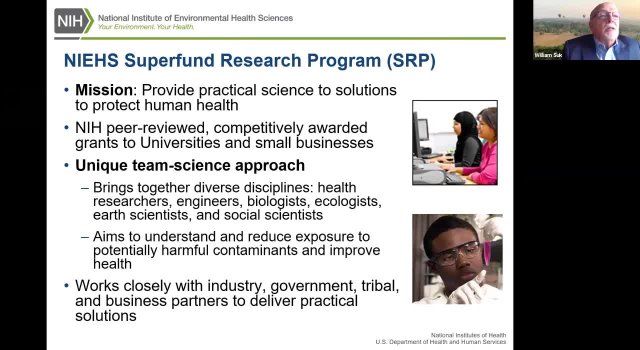 peer review, competitively awarded grants to universities and small businesses. It's a unique program And we use a lot of the word unique all the time, But the point is is that it is a unique program because it brings together a diverse group of disciplines, a very diverse group of. 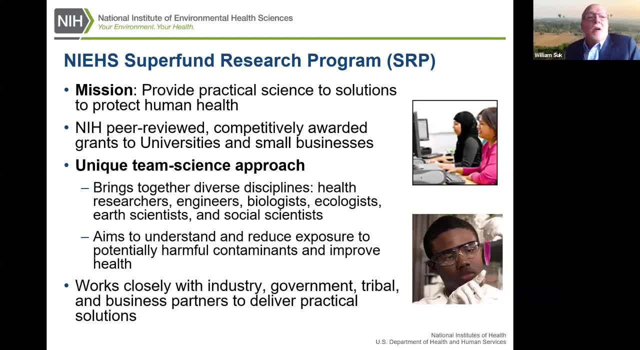 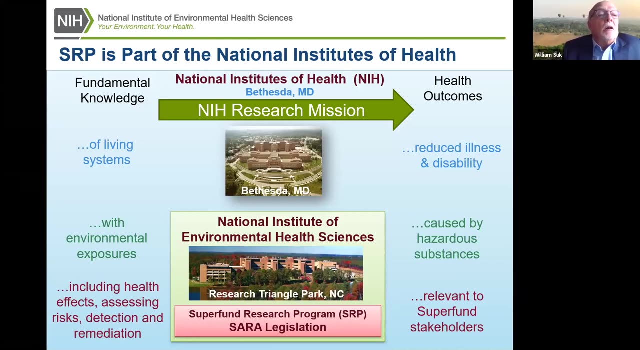 research domains of health- researchers, engineers, biologists, ecologists, et cetera, anthropologists, social scientists- and the aim is to understand and reduce exposures and thereby improve health. Next, please Thank you. So, just to put it in perspective, we are a part of NIH, the National Institutes of 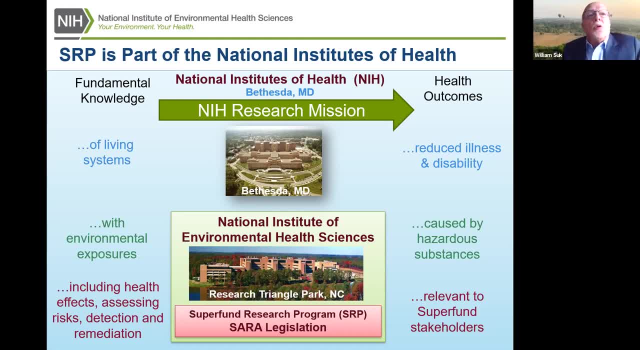 Health. we use all the policies and procedures associated with NIH. The Superfund Research Program has been in existence longer than I believe- a number like something like 10 other institutes and centers at NIH- And frankly, I consider us, and we consider us sort of a mini IC, if you will, but we are. 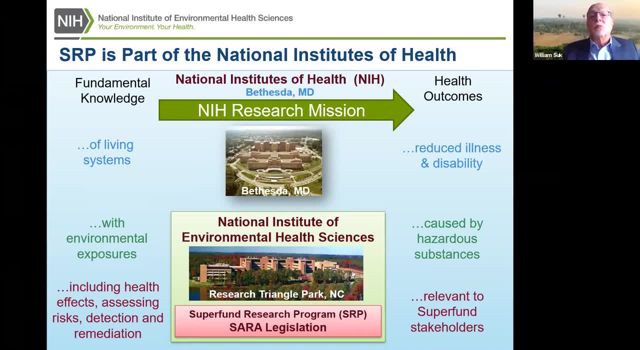 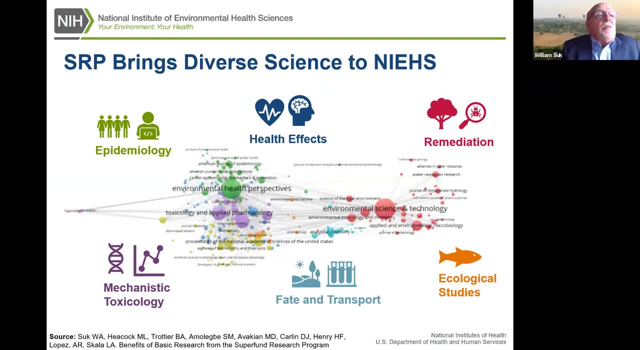 embedded within the National Institute of Environmental Health Sciences, And I'm going to go through that as to as to how that, how that works, Next slide, please. But first I wanted to give you a perspective on the diversity of the science that we support. This is a landscape map. 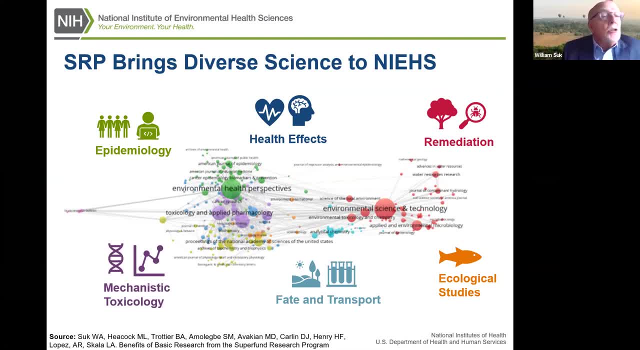 of the research that we support. The map shows journals that are funded by from research is funded by the National Institute of Environmental Health Sciences, And this is a map of the research that is funded by the program. on the left side is the biomedical research And on the 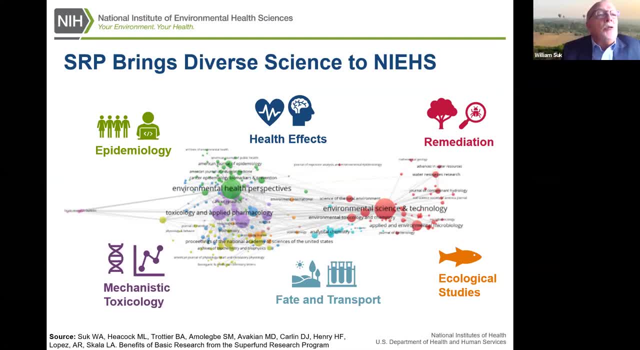 right side is environmental sciences and engineering, But you can get a very good understanding about how diverse the sciences within this program And it is the diversity of the science that is the strength of the program, because it's trying to answer questions that cannot be answered by one discipline alone. Sounds simple, But again, it's the diversity of the 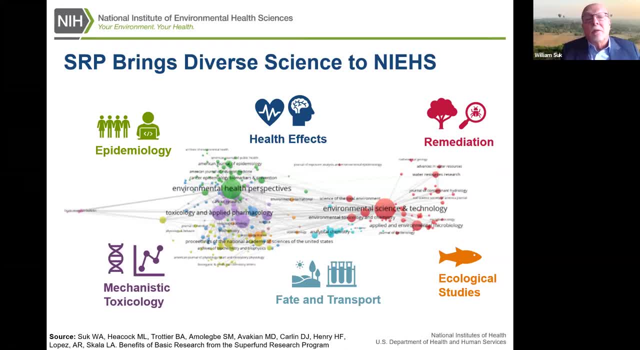 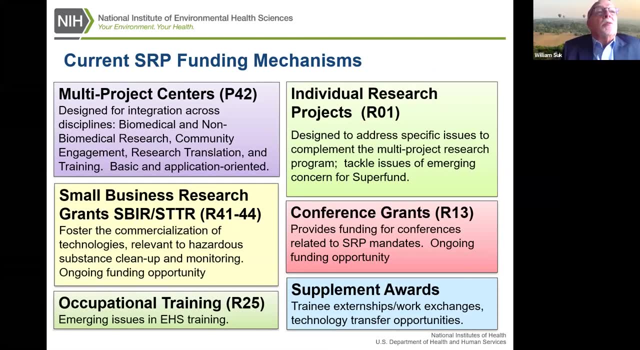 research that's happening around the world. So it's really interesting. It's a very exciting concept that we're studying, But again, if it was simple, if it was, you know if we're simple- it'd already be done. So next slide, please. So this is the makeup of the current mechanisms that 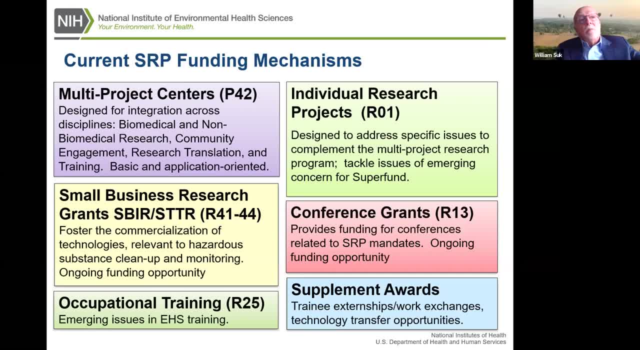 we have funding mechanisms for the SRP, The multi project centers program, the P 42. That is a unique mechanism for NIH. There is no other mechanism NIH that's like this. We do have SBA ours, we have occupational educational training, We have an R01 program, we have a conference grants. 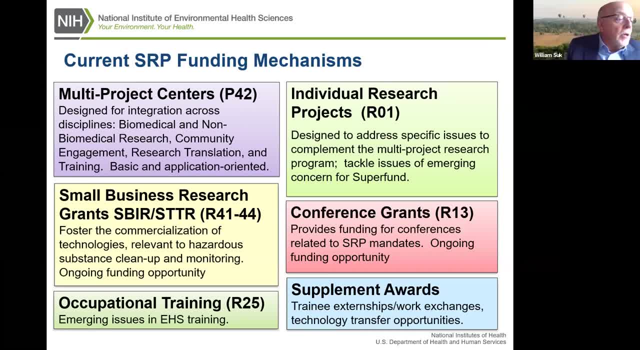 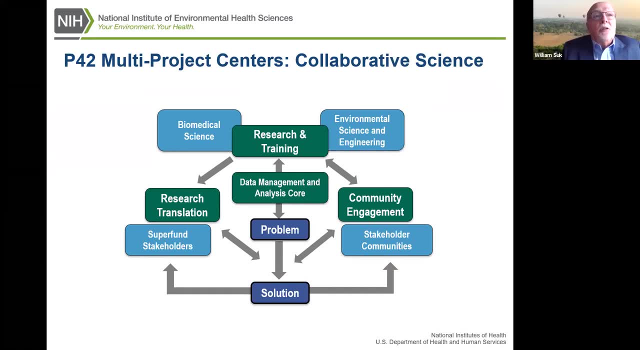 and we have supplemental awards, As I mentioned a minute ago, we adhere to all of the grant mechanisms that we can take advantage of at NIH. Next, please, So each. I'm going to focus primarily on the P42 mechanism at this time, because it really is the mainstay, the anchor of the program. 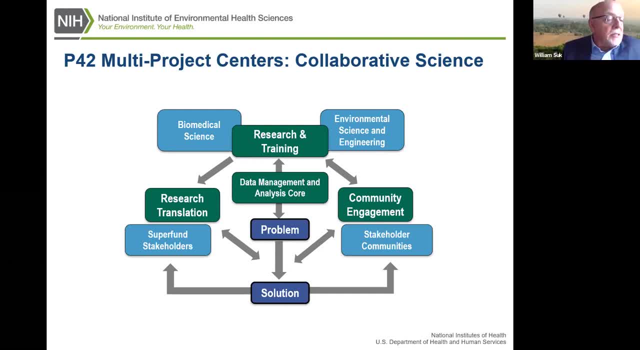 So the idea here is that this gives you- should give you- an idea about the different pieces that will come together to address a problem. You have biomedical science, environmental science, engineering. We've added over time different things like research, translation, community engagement, data science and management. 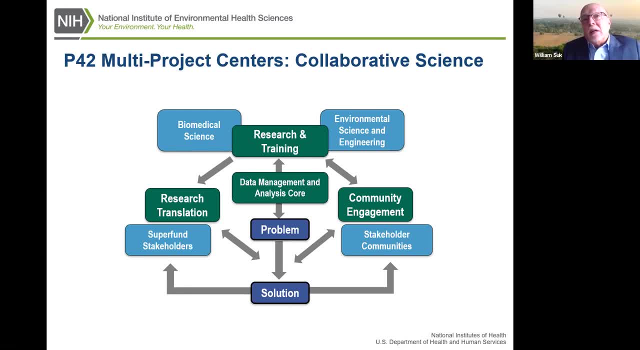 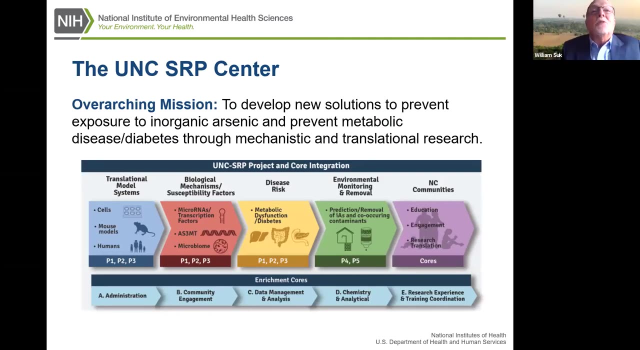 et cetera. The idea here is to develop a program that is solution oriented and yet basic in its approach, basic, fundamental research in its approach. Next, please- Now, you've already seen this slide when Rebecca made her introduction, and I smiled when I saw it because 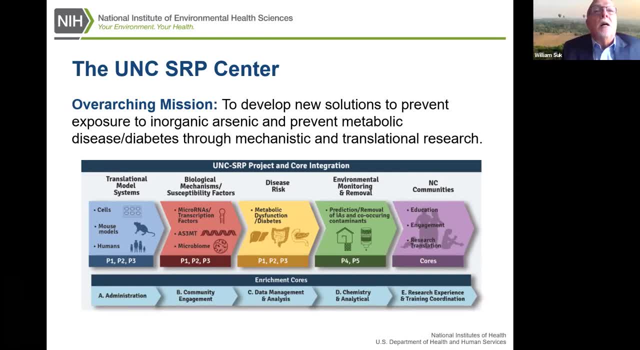 I thought, wow, you know, plagiarism is the highest form of flattery, And so I've. this is the center. It is to develop new at UNC. it is to develop new solutions to prevent exposure to inorganic arsenic and prevent metabolic diseases such as diabetes through mechanistic and 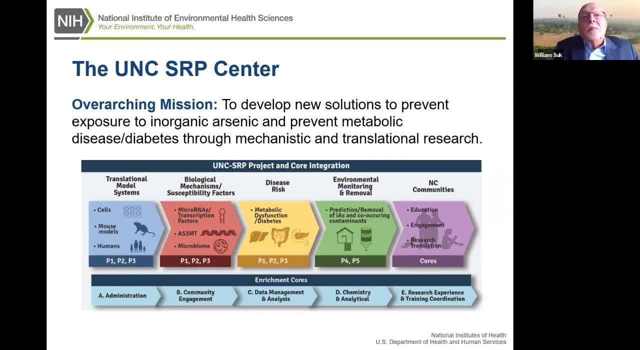 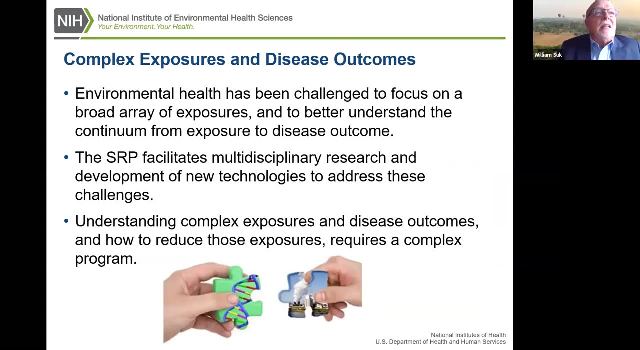 translational research. This is a great example of what I just talked about in the previous slide, about as we go on. Next, please- And the reason for having these multiple pieces is the complex nature of exposure to disease outcome. We are in the environmental health field. 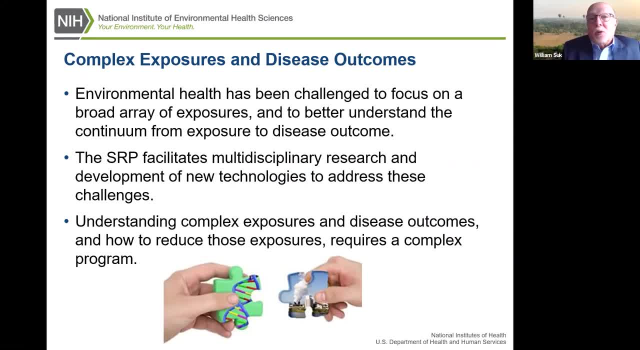 we are challenged to focus on a broad array of exposures and to better understand the continuum from exposure to disease. Sorry, I have to use my hands, because if I don't use my hands, I can't use my mouth. So the SRP facilitates multidisciplinary research. 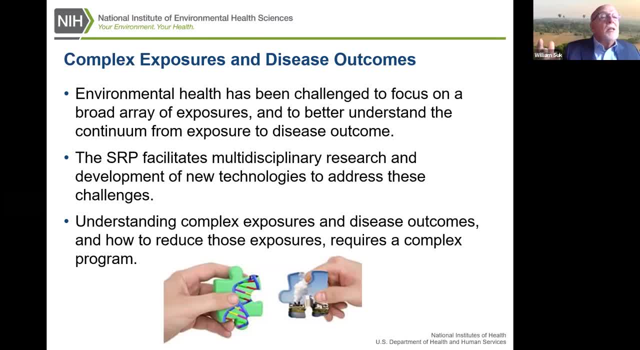 and develops new technologies to address these challenges. Having this exposure to disease continuum requires a complex program, because, I mentioned, not all programs can, not all research can address a problem on its own any longer, at least in the environmental health sciences realm. Next, please. 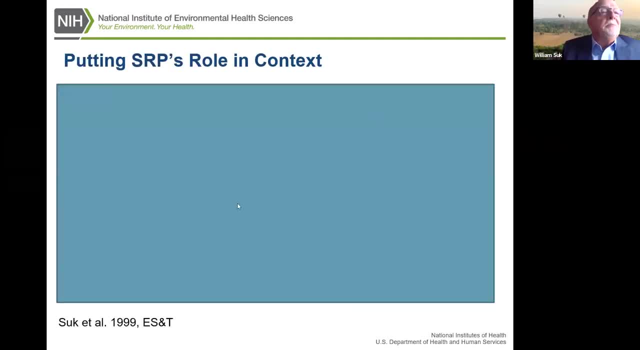 Push the button please. Okay, so don't push it too hard. So interestingly enough, I actually gave a presentation at UNC some years ago and the audience was impressed with it enough. I believe it was Mike Eken who suggested the idea, actually. 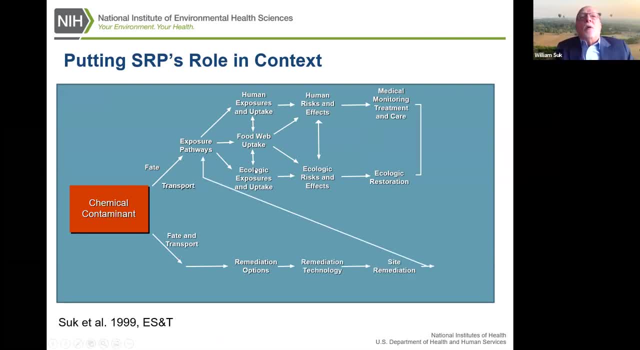 that it be published in ES&T. Now, of course, way back when we were dealing with different And it wasn't motorized like this particular presentation, but in this day and age we can do that. But what it shows is how the different pieces of focusing from an exposure standpoint of 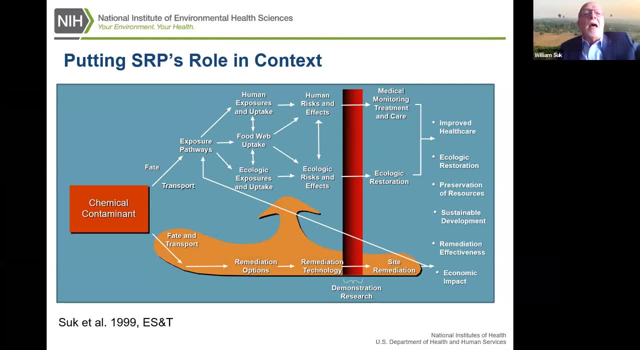 a chemical contaminant, all the way through the different risks and what one needs to do in order to remediate or understand it. And I'm going to point out that in the lower right-hand corner. as to the different areas that we are trying to focus on, one of them is economic impact. okay, 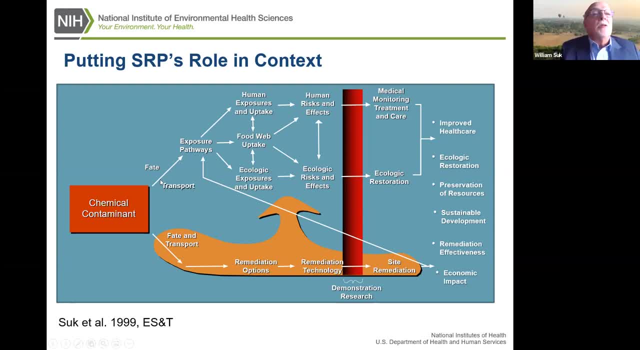 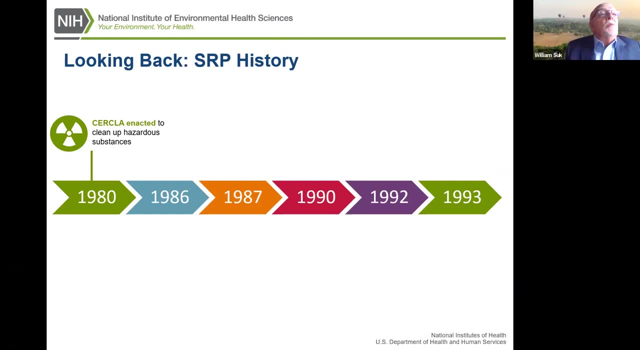 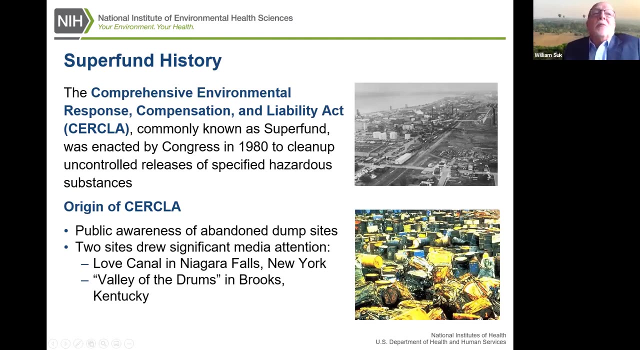 And I'll talk about that in a few minutes. Next, please. So now you're going to get a bunch of timelines. So in 1980, CERCLA was enacted. Next, please. So CERCLA is Comprehensive Environmental Response, Compensation and Liability Act. 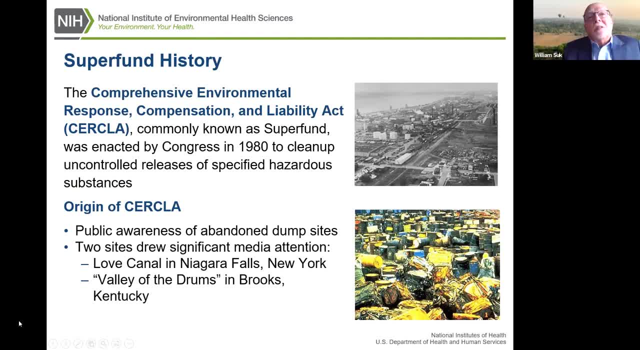 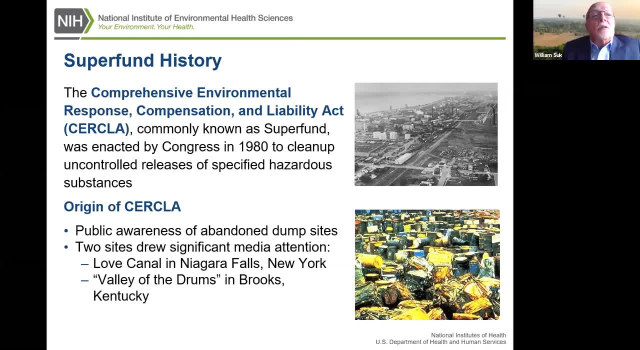 The interesting thing, or one of the interesting things about Love Canal is that it was an industrial site, a hazardous waste site, in the 40s and 50s, and then it was paved over and a community was developed there. So you had housing and what have you? 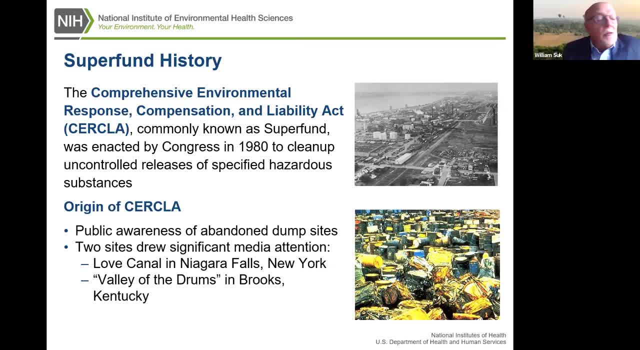 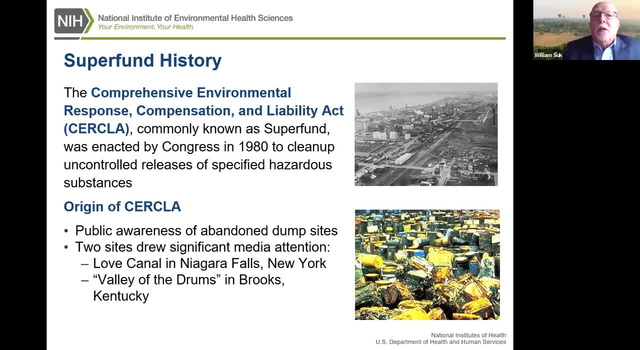 And this created a whole new community, And this created a whole new community, And this created a whole- essentially a firestorm of public opinion as to we needed to do something about this. So that's when they created CERCLA in order to clean these sites up, with the assumption that 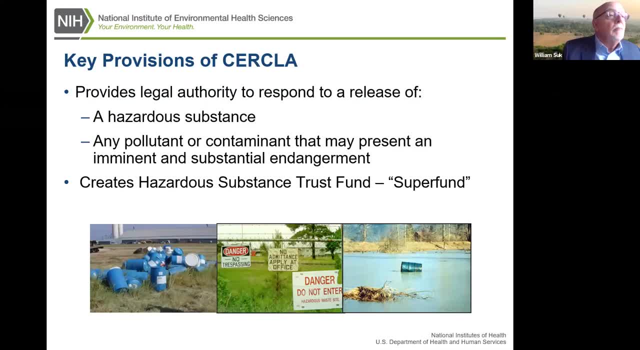 they knew what they were cleaning up Next, please. So the key provisions of CERCLA is: provide legal authority to respond to a release of hazardous substances, any pollutant or contaminant that may present an imminent and substantial endangerment. Okay, 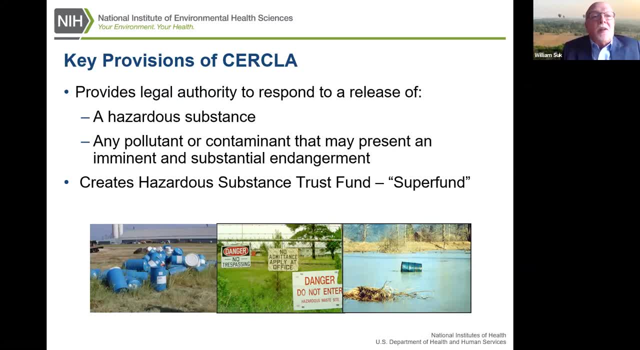 Okay, And they created the super fund substance trust fund, which has now been eliminated from Congress by Congress, and now the money for cleanup has come out of general revenue. It's not a tax on industry any longer. Next, please. 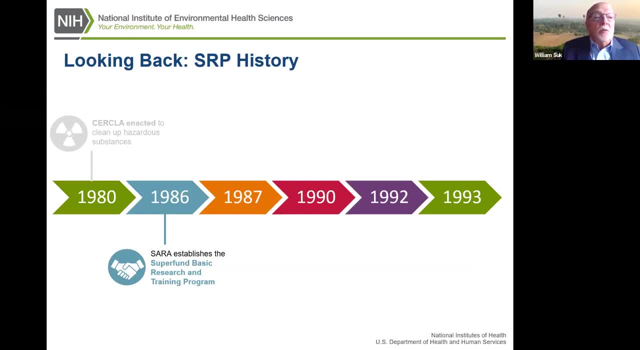 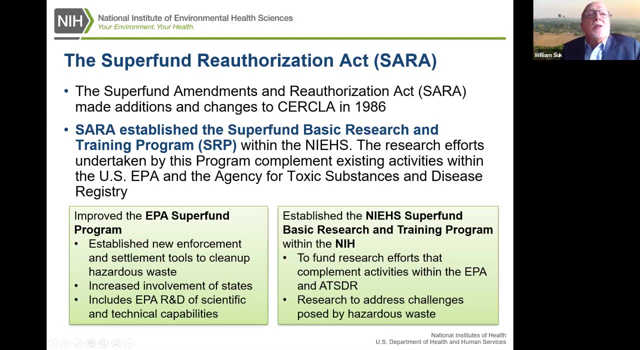 So in 1986, CERA was established. Next, please, Next, please, Next, please. So CERA is the Super Fund Amendments and Reauthorization Act which made additions and changes to CERCLA And CERA, established the Super Fund Basic Research and Training Program- otherwise we've shortened it to SRP within the NIEHS. 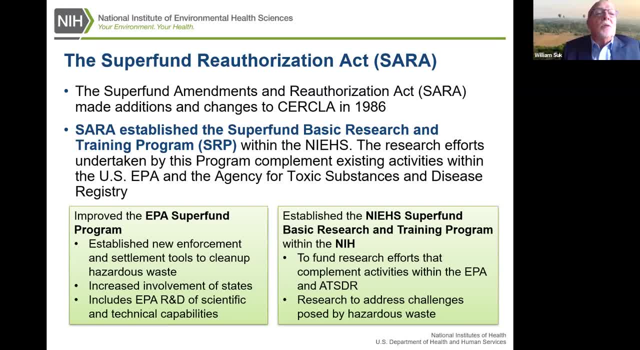 Okay, Next, please, Next, please. So the whole idea here was to establish a research program to be supported by unoscientists- Next please, Next please. superfund dollars, essentially to look at issues that are fundamental, because they recognized that. 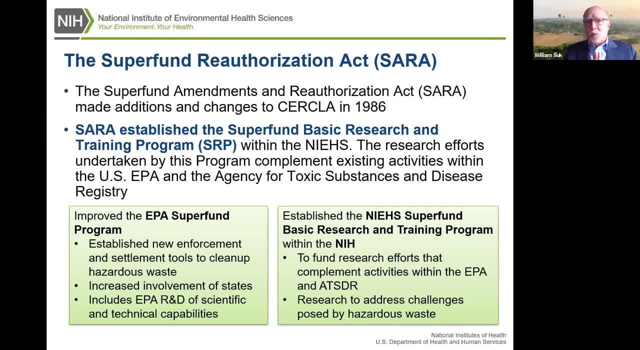 it was important to say: oh, what kind of questions do we need to have answered in five or 10 years from now? Nothing take, you know, basically EPA and regulatory agencies, which is perfectly which is what they do. is they address problems today? The question is, what problems are they? 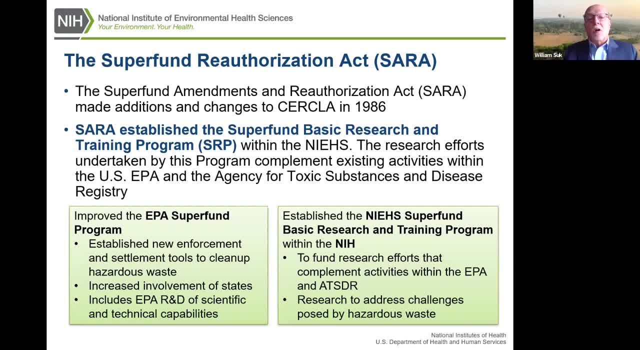 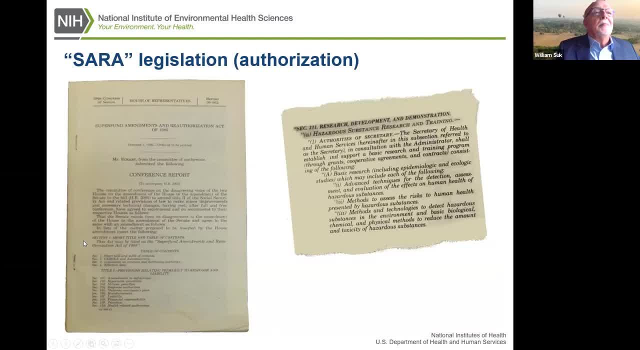 going to have tomorrow that need to be addressed And that's where superfund, the SRP, comes in Next. please Thank you. So this is, believe it or not, the entire legislation for the superfund research program. okay, It is essentially a page and a half. However, what it does is it gives. 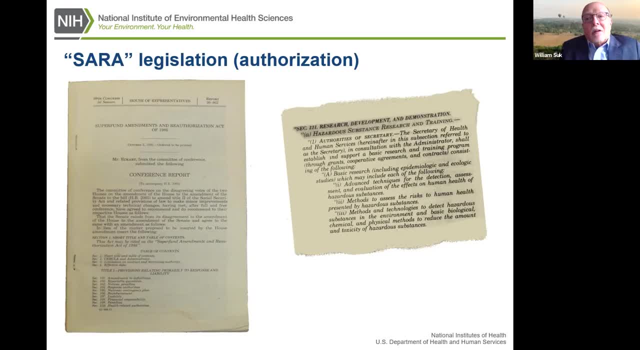 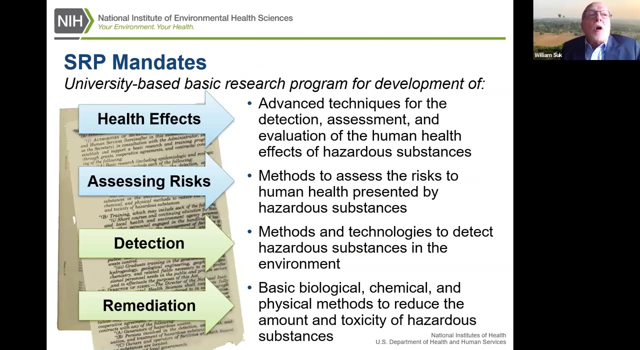 NIEHS a lot of flexibility. There are certain things in there that are very important. Next, please, These are the four mandates that we adhere to. This is the driving force behind the entire program. It is we adhere to these in whenever we have to make decisions as to who we're going to support. 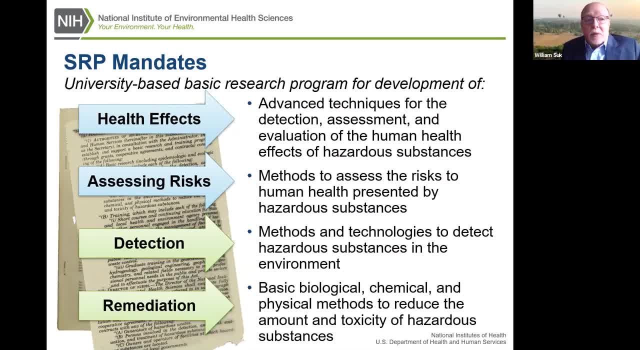 And we also look at things from the standpoint of relevancy based upon these four areas. So, advanced techniques for detection, assessment, evaluation of human health of hazardous substances. methods to assess the risks to human health presented by hazardous substances- The reason why I'm emphasizing that Methods and technologies to detect hazardous substances in the environment. 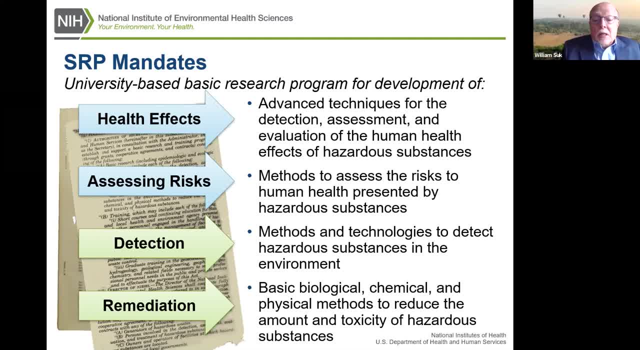 and basic biological, chemical and physical methods to reduce the amount and toxicity of hazardous substances. Nowhere in the legislation does it use the word hazardous waste, use the word hazardous based substance, which gives us a broader mandate. The other part to this is it also is not a site. 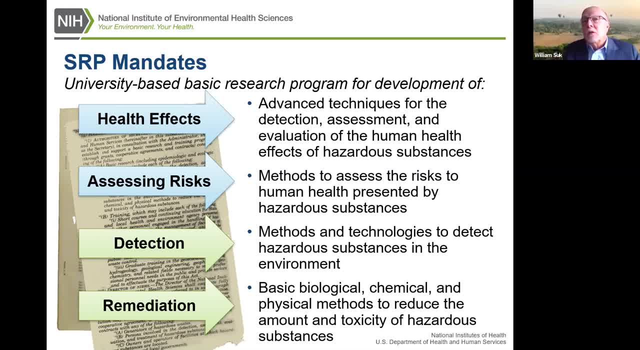 specific program because the research that's done at UNC needs to be generalizable and applicable to problems of arsenic in other parts of the country. Okay, And the unique thing about these mandates is that is number four: remediation Size uncovered Terrain. 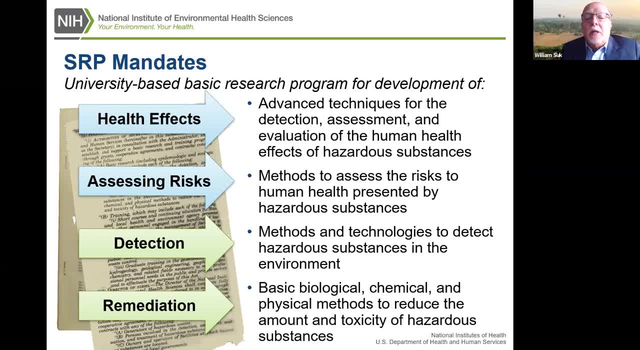 resource operation, more good service and weight capacity and health industry. Some of these impacts still need to be looked at in the second half or the third half of a year, So I'm quite optimistic on today. In addition, there is the real Zurich換 therapy program on hand. We have Franklin機. 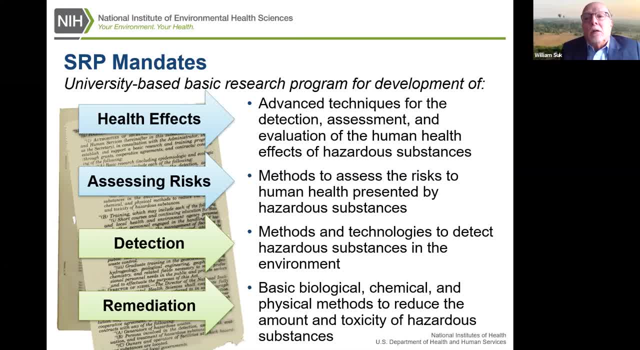 remediation: Nowhere. NIH does not fund research like this. In fact, we're one of the only organizations that does support basic, fundamental research with regards to remediation. I know EPA does and DOE does and the Department of Defense does. 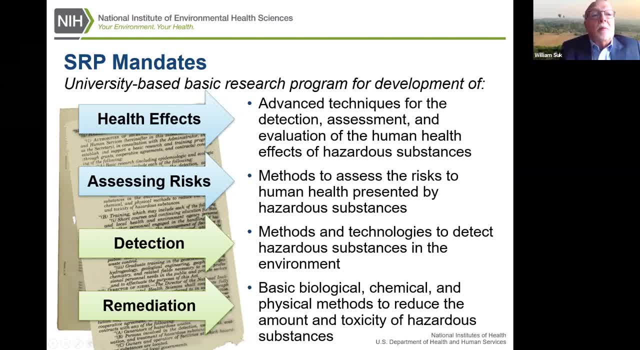 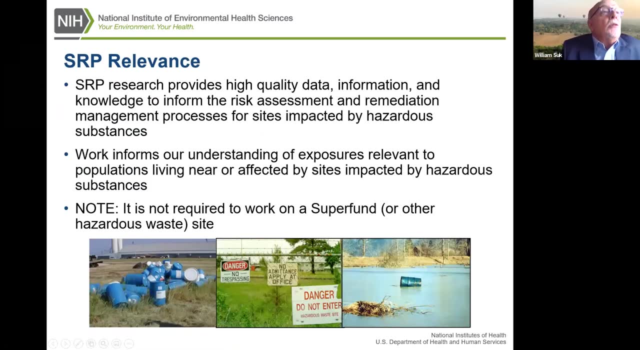 as well as the National Science Foundation, But we're the only program at NIH that does that and we're the only program that requires people to address these areas within their application when they try to get support Next, please. So the relevance provides, the research provides. 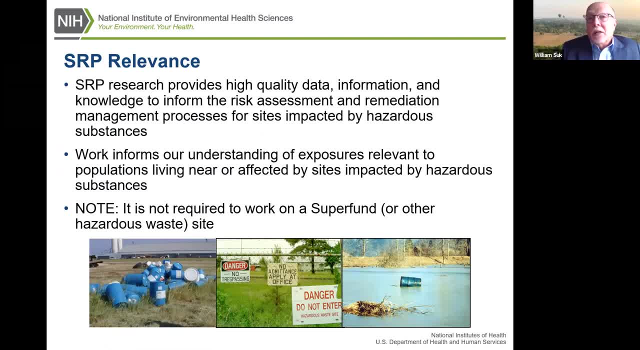 high-quality data, information and knowledge to inform the risk assessment and remediation management processes for sites impacted by hazardous substances. Now again, it's not site-specific, however, So we work to inform an understanding of exposures relevant to populations living near or affected. 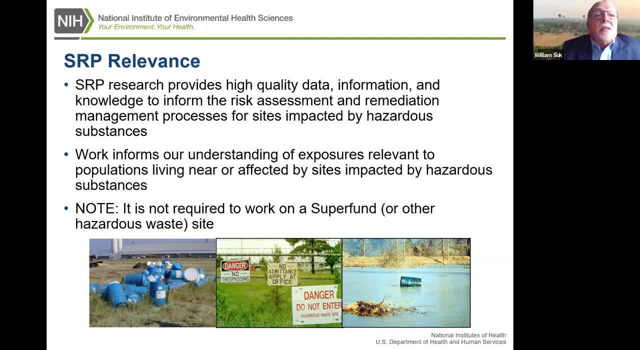 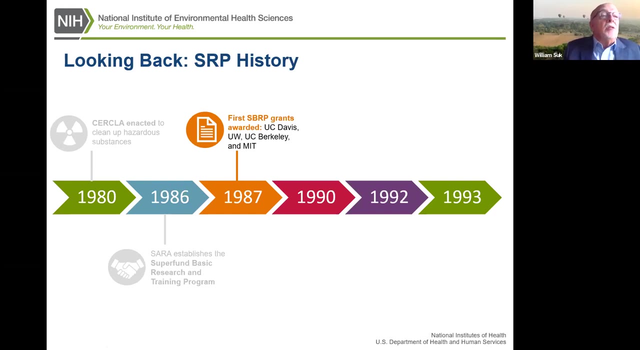 by sites- And again I note that it is not site-specific and we have a broader mandate, essentially, than by just using the word hazardous substances Next, please, Okay, So, like I said, we were established in 86 under Sarah And then in 87, we made our first awards. 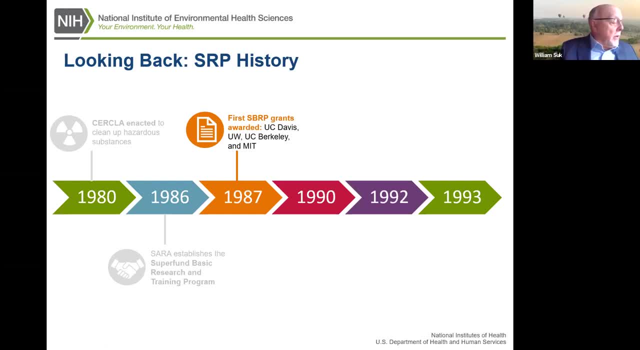 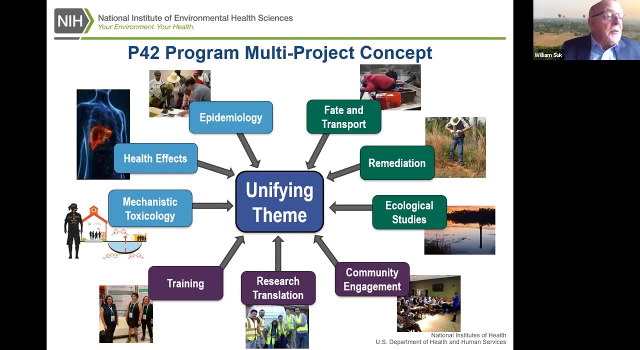 to those four organizations. We had a whopping budget of $3 million. Next slide, please. But the whole idea back then and today is pretty much the same and that is we're trying to bring. we are bringing multiple, we are bringing more disenfranchised disciplines together under a unifying theme to address problems. 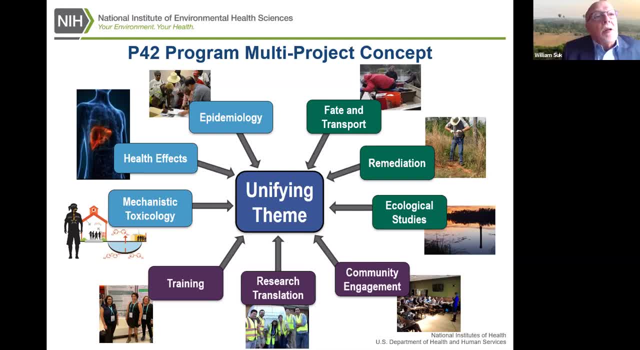 that cannot be addressed singularly And they have to- and each center has to do it in an integrated by. They have to be able to demonstrate that they are communicating and talking to each other and being able to actually build in training and research, translation and community engagement. I get. 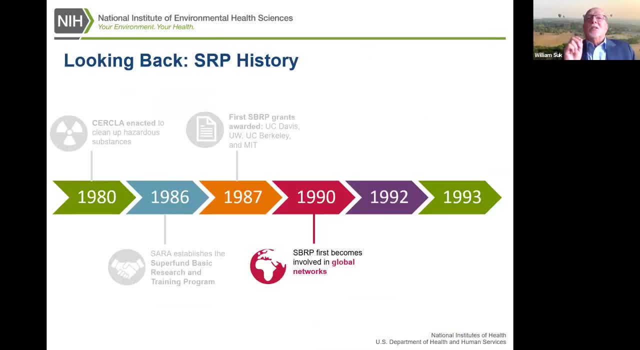 to that also. Next, please, I'm going to not shift gears, but just to give you a broader perspective as to what happened then, because it also has to do with some things that happened later on. Everything is kind of interconnected, just like the whole program is. So we became global in 1990.. Next slide: 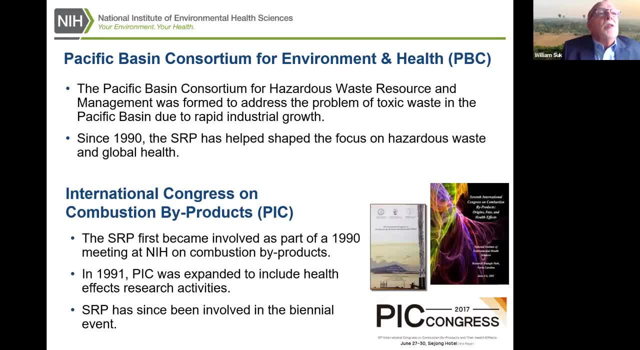 We found ourselves working with the Pacific Basin Consortium for Hazardous Waste Resource and Management, which then became the Pacific Basin Consortium for Environmental Health, Environment and Health, PBC. It was based in the East-West Center in Honolulu. The issue is that exposures to hazardous substances is not only a US issue Also. 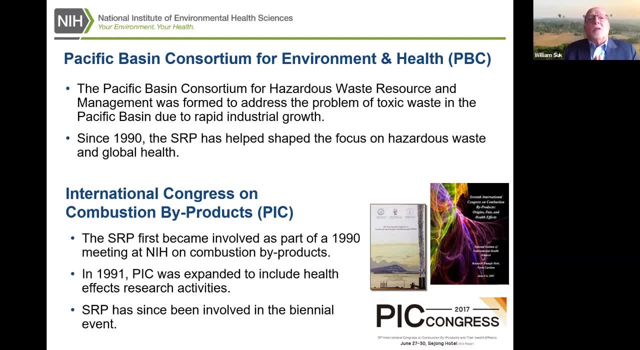 research that takes place in other parts of the world can be directly applicable to problems that we have here in the United States, And I'll cover that in a minute. We also have been supportive of the PIC conference, the International Conference on Combustion. 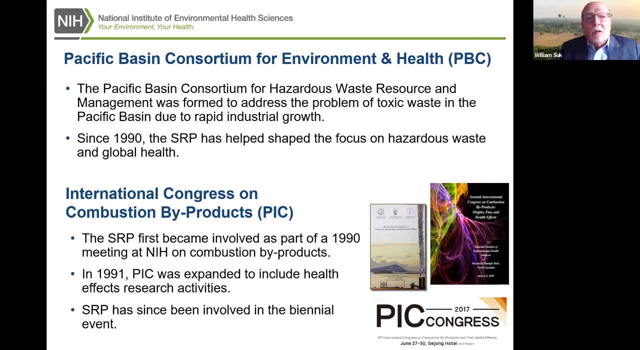 Byproducts. It started out primarily as an engineering organization looking at combustion byproducts And then within a year or so, we got involved And the poster that you see were the seventh Congress that was actually hosting the PIC conference, And then within a year or so, we got. 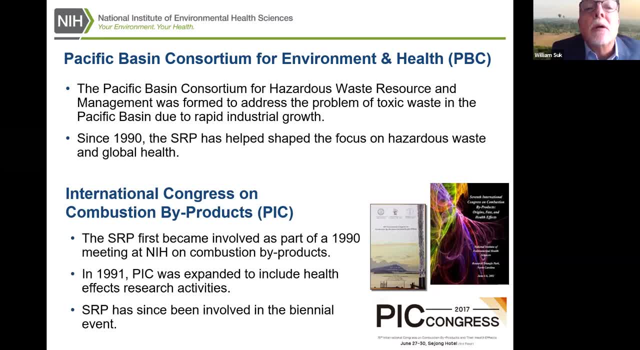 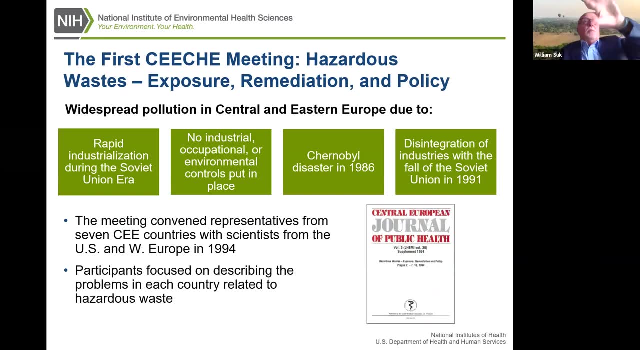 involved and hosted and held at NIEHS 2001,. it looks like, And so that's one more slide. One more thing, Next slide, please. So the other part to this too is that Pacific Basin Consortium and PIC is global in that it looks at combustion byproducts, But we also started looking at 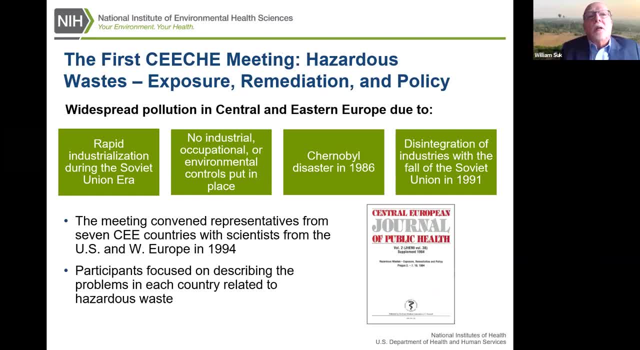 what the issues of widespread pollution in Central and Eastern Europe are, And we also started looking at what the issues of widespread pollution in Central and Eastern Europe are, And we also started looking at what the issues of widespread pollution in Central and Eastern Europe are, And we also 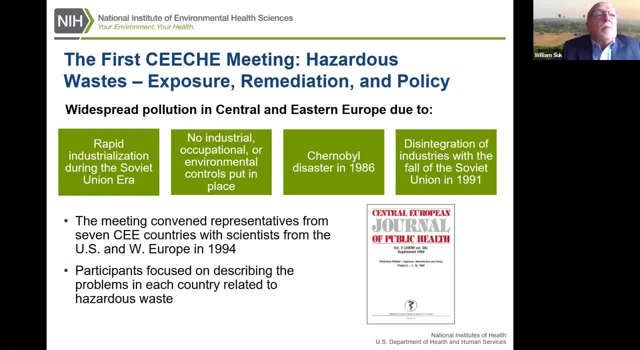 Europe due to these issues. I mean there was incredible rapid industrialization during the Soviet era. no controls whatsoever. There was, like it says, no industrial, occupational, environmental controls were in place during the Soviet Union. Then they had Chernobyl. 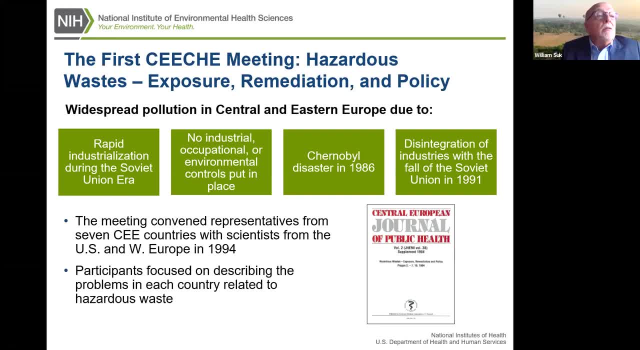 and then the Soviet Union dissolved and you had some real issues with regards to populations being exposed to an incredible amount of things, and so we got involved- And when I say we, I mean our grantees- In each one of these situations. I'm just using these three as examples in each of 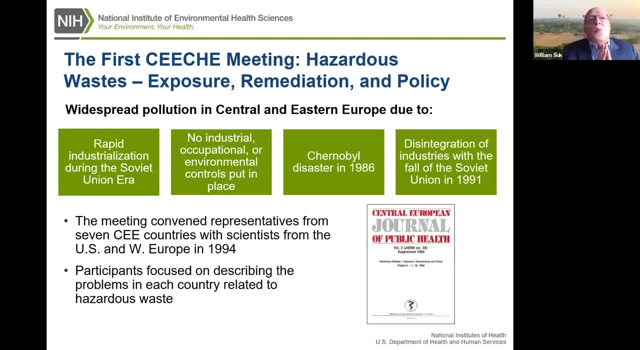 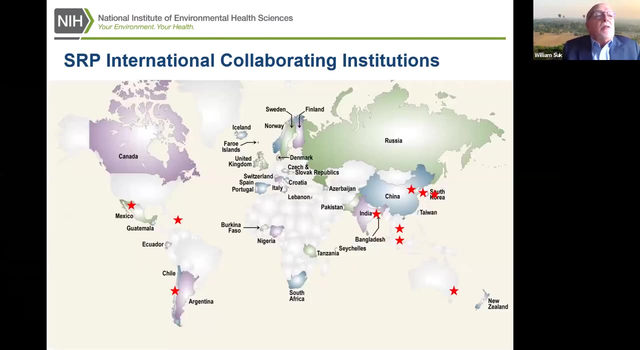 these situations, of these organizations. we have researchers who have an interest in that part of the world for one reason or another, and the research that we support here in the United States is then translatable and transportable to other parts of the world. Next slide, please. So these are the areas that we are presently working elsewhere in the world. 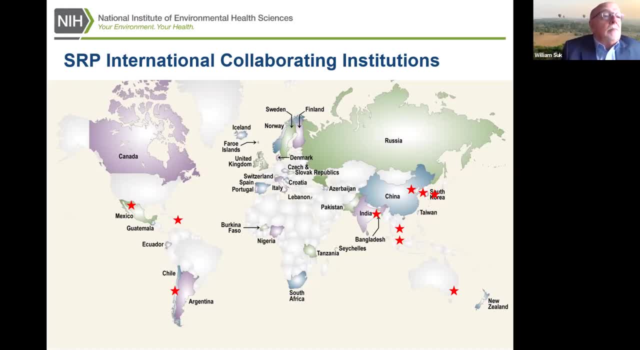 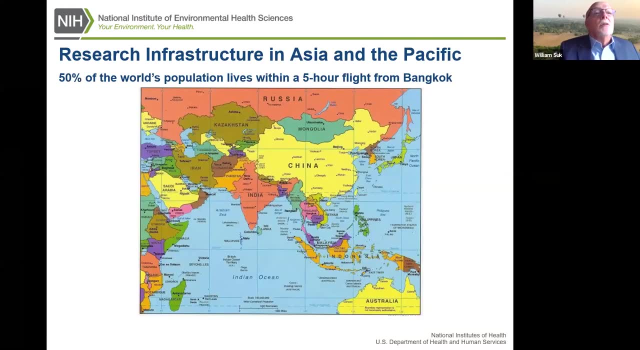 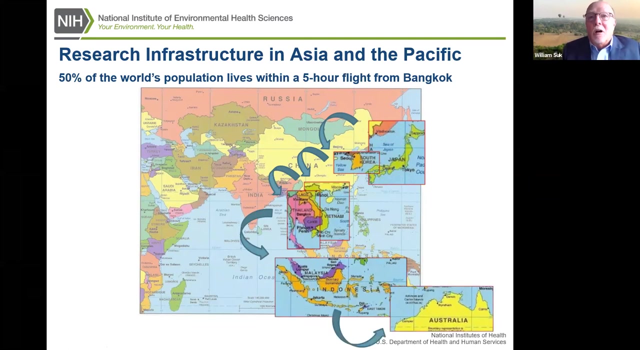 and there's research going on. I'm going to cover a few of this in a minute. Next, please, Okay, hit the button. Here we go, Okay. So this demonstrates that in South and Southeast Asia there is an incredible research infrastructure that is available for understanding the links between exposure to. 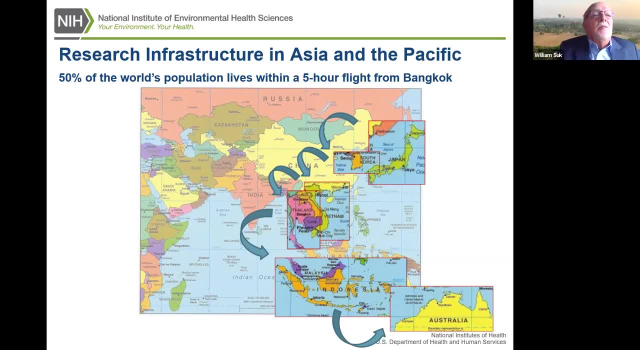 disease. I will also indicate that if you put a pin in Bangkok, okay, and you fly five hours in a circle, you will cover. well, you cover most of China and India and a little bit of Japan and the tip of Australia and most of Indonesia, Malaysia and everything in between, but that's. 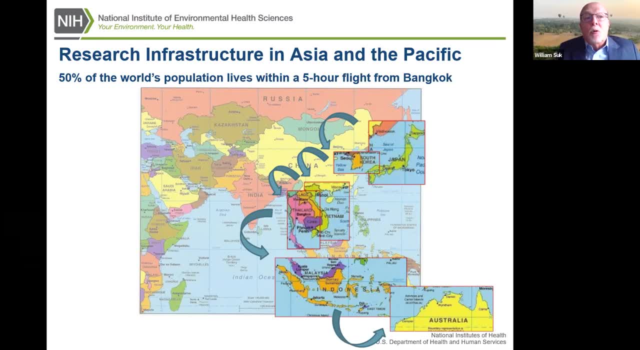 half the world's population. There are more people in. there are twice as many people in India as there are in all of Africa. That does not mean to diminish the exposure issues and the disease issues in in Africa. it just demonstrates that this is the central point. this is where the large 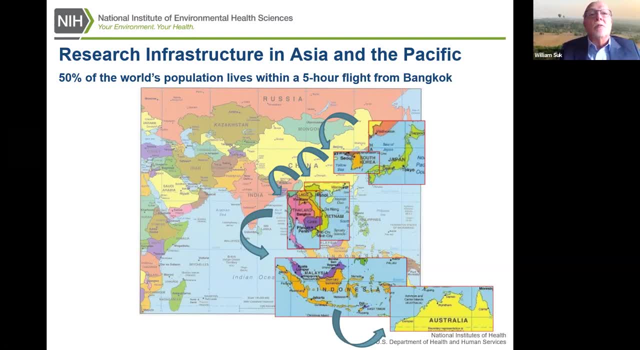 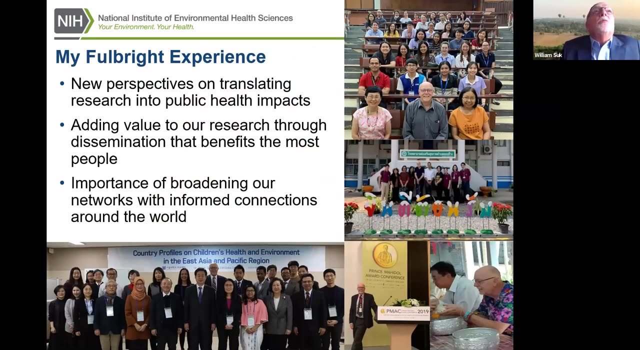 portion of the world is, and this is one reason why I had a keen interest in it for one reason or another, and so the next slide is a little bit self-serving, but I'm going to tell you anyway. in from January, from December of 2018, until June, the end of June of 2019- I was a Fulbright global. 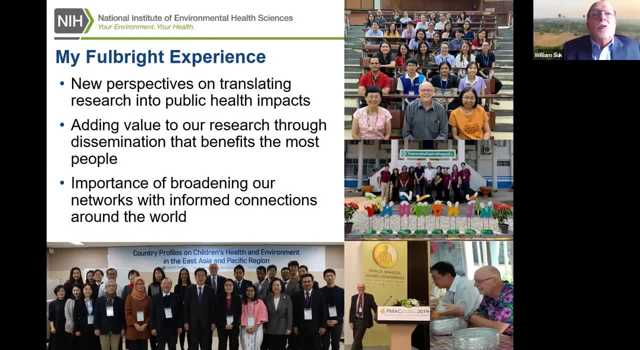 scholar at the Chulaborn Research Institute and Mahadol University in Bangkok, Thailand, but I did find myself spending time in South Korea, as well as all kinds of all other places in Thailand, as well as Vietnam. the focus of it was on children's environmental health and developing research infrastructure. 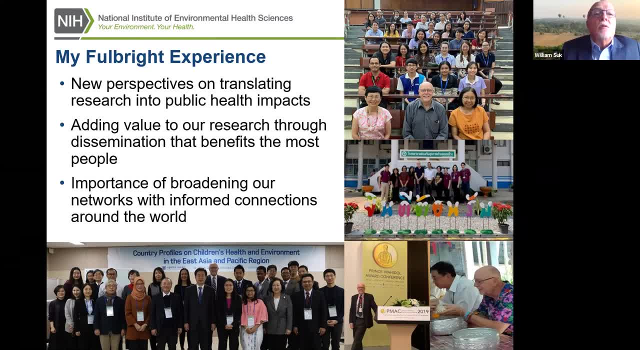 in the on that issue with different universities and organizations, public and private, to gain a broader understanding of how to be able to mentor, how to be able to teach, how to be able to do things that are important for in this world and in the future, and I think that's what I'm going to talk about today. 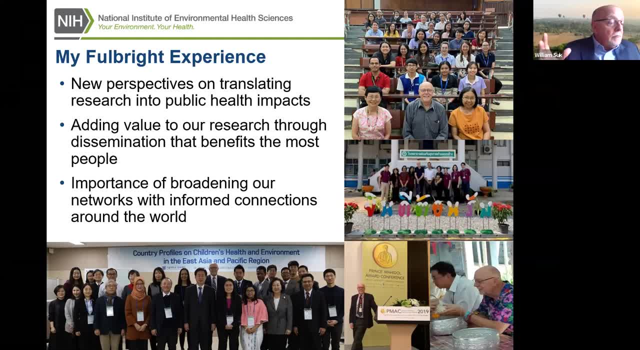 and I think that's what I'm going to talk about today, and I think that's what I'm going to talk about today in this case: children's environmental health. the whole one of it was to be able to move the science forward in many ways, and 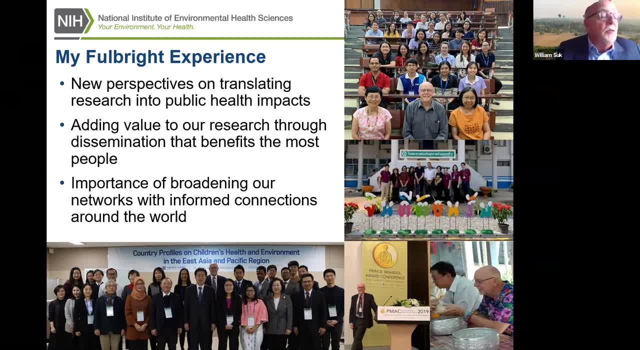 we'll talk about children's environmental health in a few minutes, but the point is is that this was a wonderful opportunity and it made for an important way of actually taking the research that you all do, that the research program at NIEHS and NIH does, to be able to do research. 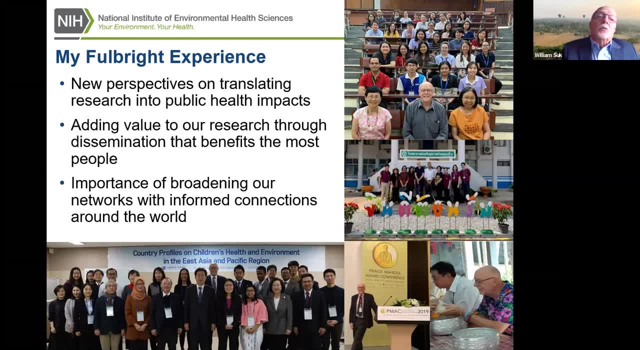 that you all do, that the research program at NIEHS and NIH does to be able to do research in order to take it to other parts of the world. I could not have done any of this had it not been for having been involved with the Superfund Research Program for us at all. 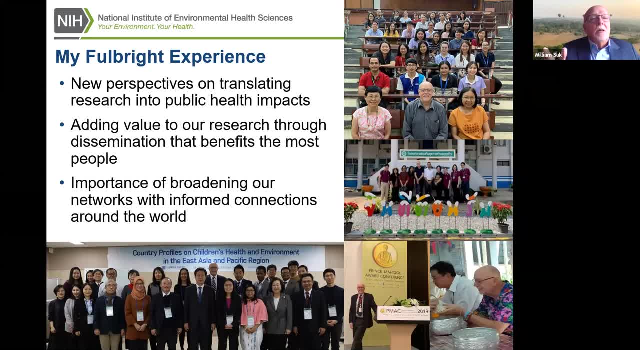 Because the whole idea again is to be able to develop research, to be able to translate the research that we are doing over there and take the research that they are doing over there. that is repli- to be able to translate the research that we are doing over there and take the research that they are doing over there. that is repli-. 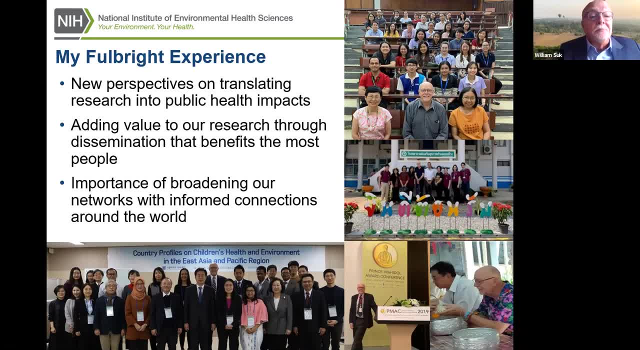 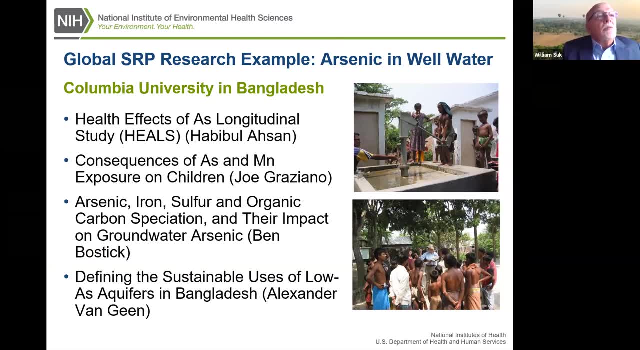 to be able to translate the research that they are doing over there and take the research that they are doing over there. that is repli- implenable to what we're doing to us Next, please. So I do want to give three example- two examples or two university examples. 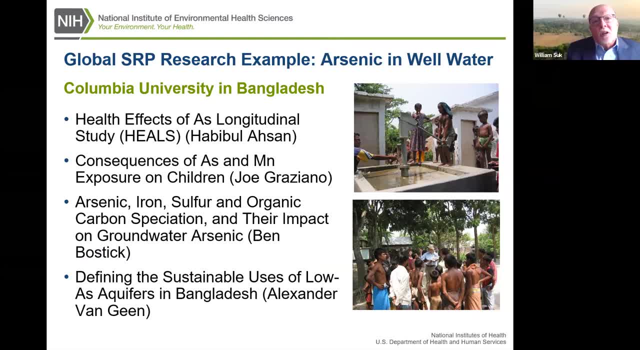 so I do want to give three example- two examples or two university examples that deal specifically- and I've chosen Arsnik because UNC centers has Arsnik. but there's a longitudinal study. this is in Bangladesh, looking at, looking, looking at over 30也是. 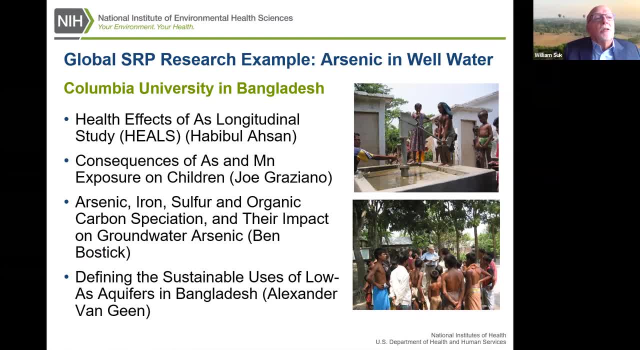 30,000 people in a part of Bangladesh that are highly exposed to arsenic, as well as manganese. If you look at the different research topics areas, you realize that it's not just epidemiology and it's not just health effects of exposure to children. It's also coming up with ways of 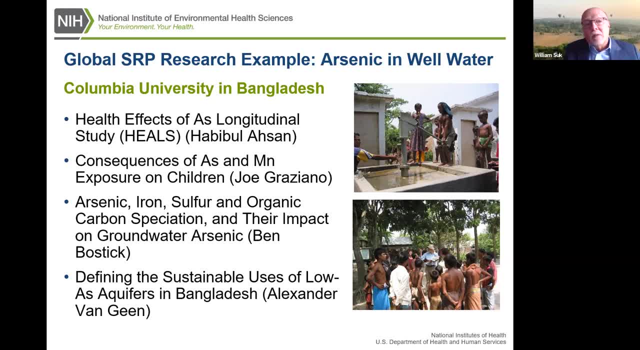 understanding how arsenic has arrived, has gotten into the groundwater, and how to be able to actually come up with ways to reduce those exposures in arsenic. But one thing I will also mention here which I found interesting, which I think you might find interesting, is that 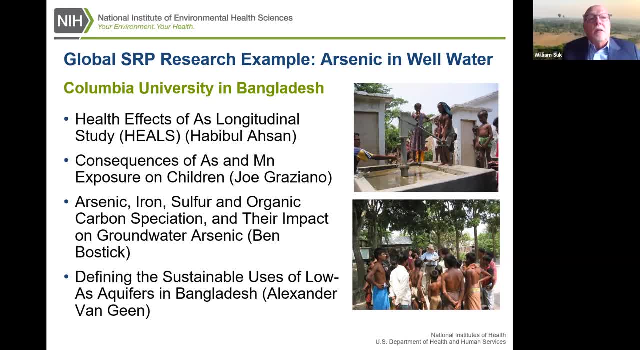 Dr Graziano at Columbia. he started working with the Chula Bone Research Institute and started doing studies that essentially replicated a lot of the work. Oh, it was also the exposures part. It was supported by Japan and the exposure was done by the Gwangju Institute of Science and 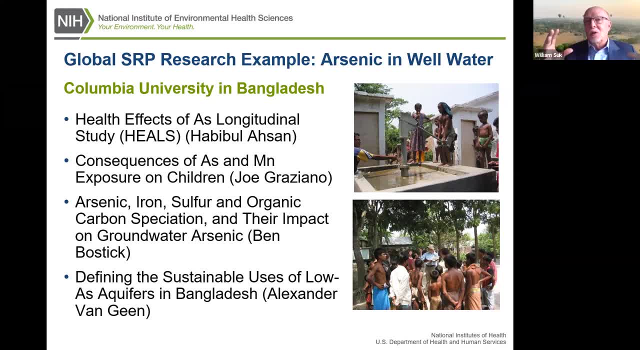 Technology in Gwangju, South Korea. So you had this incredible network of people coming together to look at arsenic in North Vietnam, And the interesting thing is that a lot of the studies, or most of the study, was actually a replication of the study that Dr Fry had done as a postdoc. 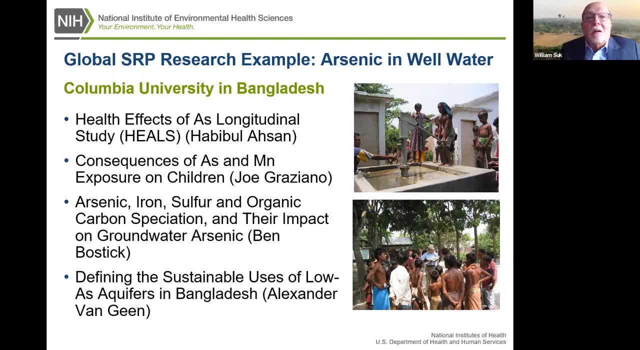 when she was at MIT, that she had done a lot of the work that Dr Graziano had done In Southern Thailand. There's a whole story as to how that came about, But what I'm getting at is that the issues that they are having over there are some of the same issues that we are having. 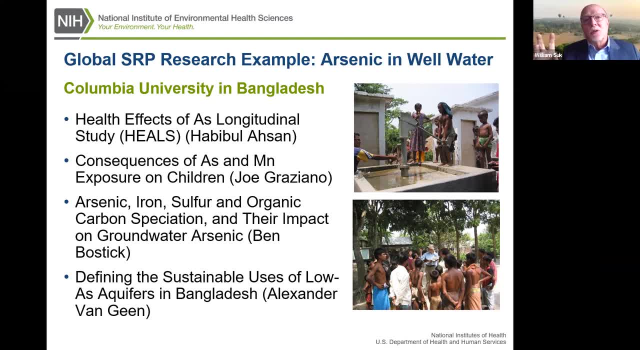 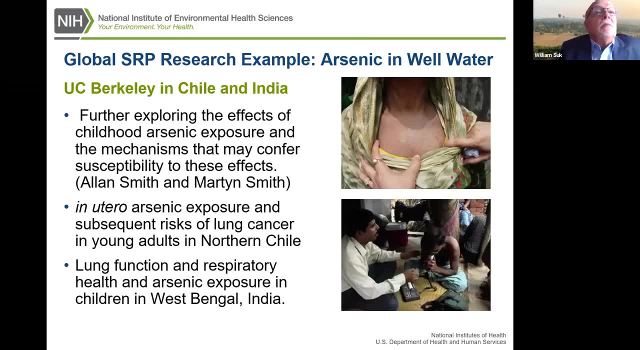 here And it's so incredibly important to be able to take the research and translate it back and forth. back and forth Next, please. So the other example- again arsenic- focuses on the work that UC Berkeley is doing in Chile and in West Bengal, India. Work in Chile has been going. 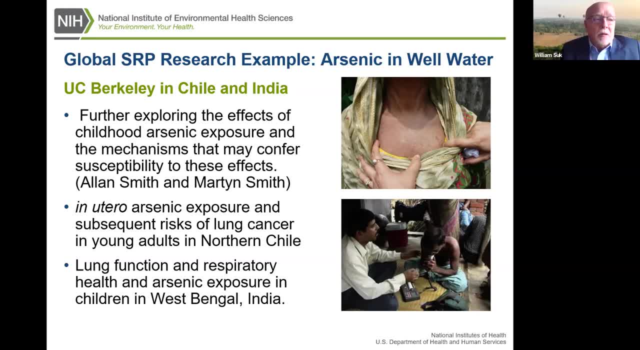 on for a long time under the under the- primarily initially under Alan Smith- and looking at childhood arsenic exposure and mechanisms that confer susceptibility. It turns out that a lot of the studies that Dr Fry and Dr Graziano have done have a lot of resistance. Some people 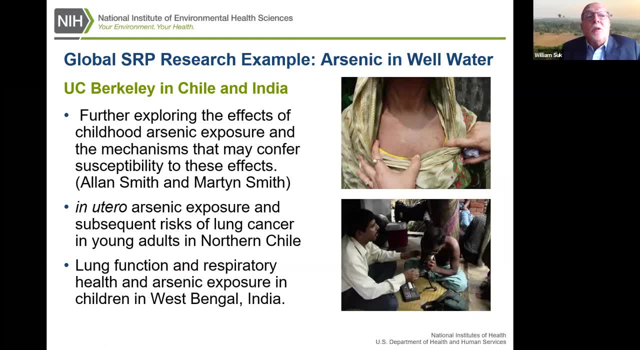 became resistant to those high levels of arsenic And it was interesting in that there was also in utero exposure to arsenic that resulted in subsequent risk for lung cancer later in life. So these are all important studies that we put into that we that we can actually use in order to get a 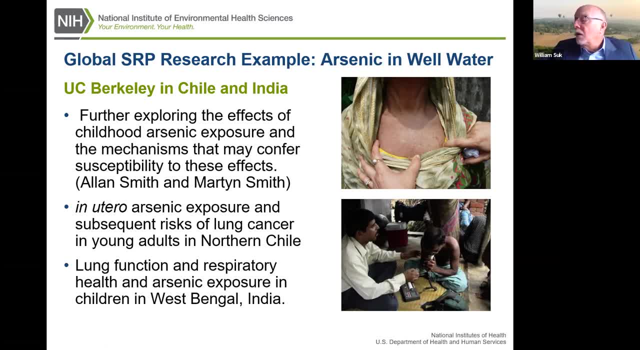 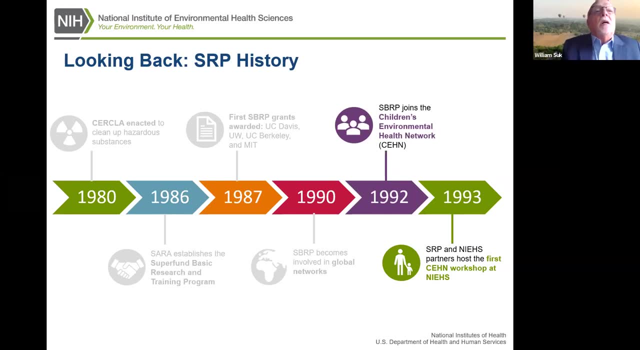 better understanding, and not just get a better understanding, but also create a better understanding and come up with ways to, to to reduce exposures. Next, please, All right, I got to move along, So we joined the Children's Environmental Health Network through an interesting part- This was back. 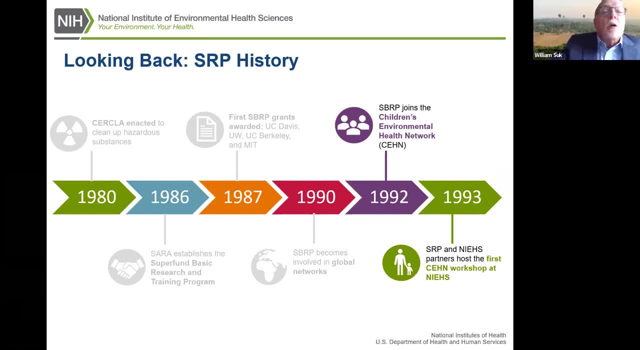 when there was community engagement- excuse me, in community outreach rather than community engagement- within the program, And we worked with them through our program at UC Berkeley and we also held the first Children's Environmental Health Workshop held at NIEHS. So the Superfund. 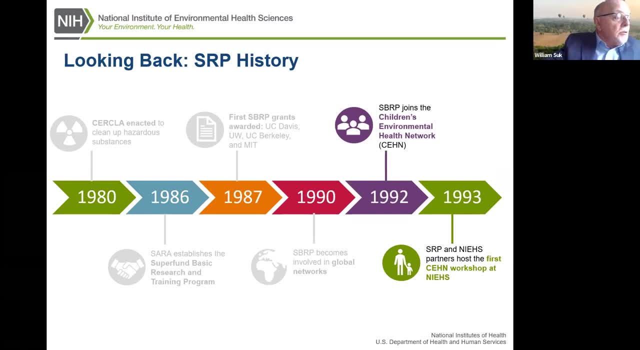 program has been involved in this for a very long time. Interestingly, between 1992 and 1998, we were intimately involved in EPA's national agenda to protect children's health and from environmental threats that was signed by President Clinton Next, please. 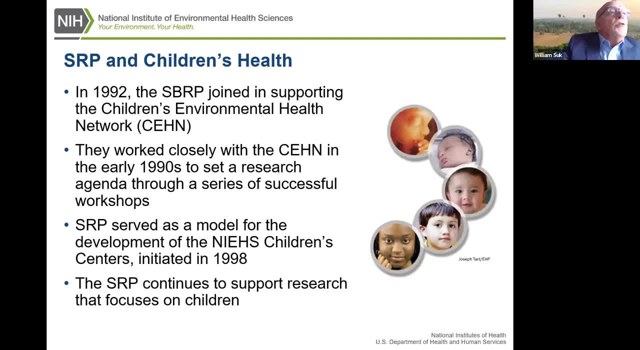 So this is a little. a little thing on the Children's Environmental Health Network. It used to be in Oakland, California. It is now in Washington DC. The director is now NC Witherspoon and it's a very good organization to to look at how to be able to protect children from. 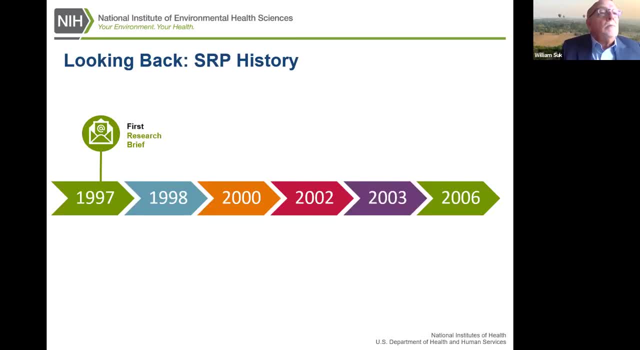 environmental contaminants Next, please, Okay. So back in 1991, there was a very, very, very large, very long, very, very high rate. of 1997, we did our first research brief. Next, Since that time, we promote SRP findings. It's one thing. 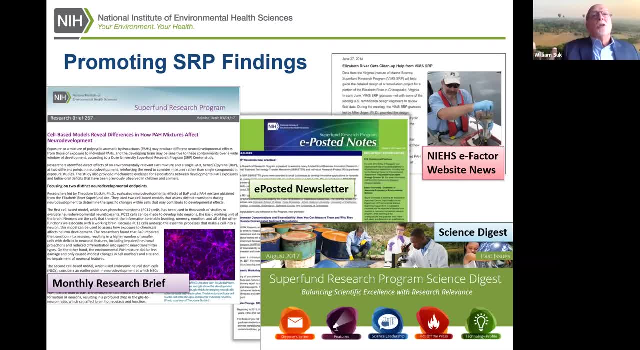 to be able to publish in high caliber, peer-reviewed journals. There's nothing wrong with that. That's great, But it's also important to be able to reach as many people as you possibly can, doing different ways, using different sources and different approaches, And these are some of the 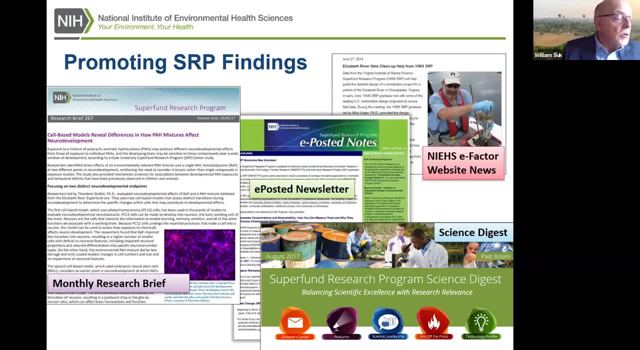 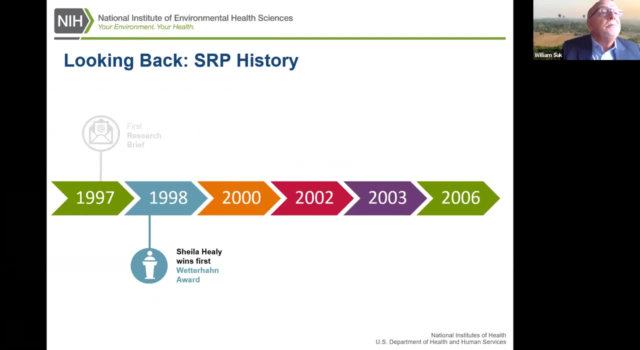 approaches that we have come up with. So we do research briefs. So far we've done 312 research briefs. They come out every month And it reaches more than 11,000 people worldwide. Next, please, So in 1991,. 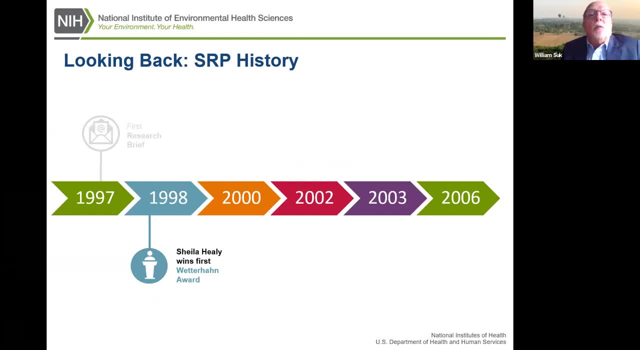 after the death of Karen Wedahan, we established the Wedahan Award And that was for young investigators, pre-docs and post-docs, who would basically do outstanding research but also do different things with the community, do mentoring programs and are demonstrating. 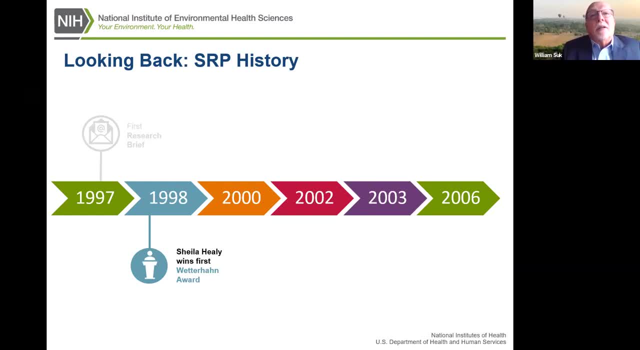 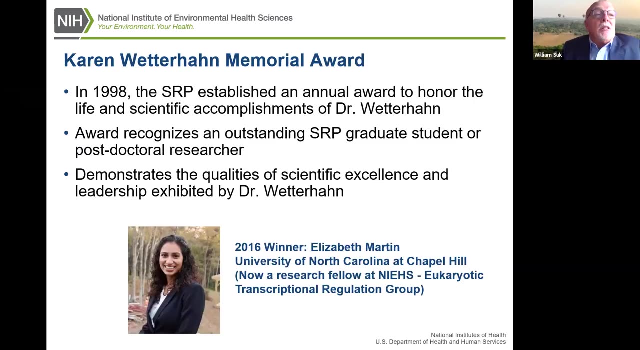 Karen's legacy. essentially, She was a very good friend and a colleague And she was an outstanding researcher and a very nice person. Next, please. So, as mentioned, the Wedahan Award demonstrates the qualities of scientific excellence and leadership exhibited by Dr Wedahan, And the 2016 winner is Elizabeth Martin, who is now a research fellow at NIEHS in the eukaryotic trial. 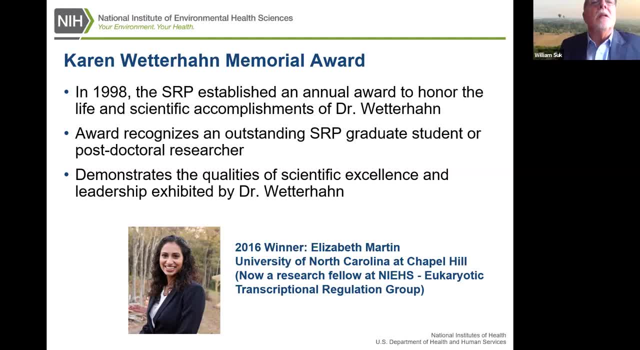 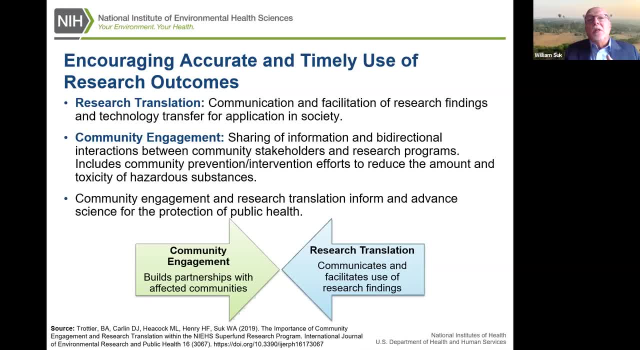 And the 2016 winner is Elizabeth Martin, who is now a research fellow at NIEHS in the eukaryotic trial. And the 66 webinar that you're focusing on to be well informed, so that they can make informed. And the 66 webinar that you're focusing on to be well informed, so that they can make informed. 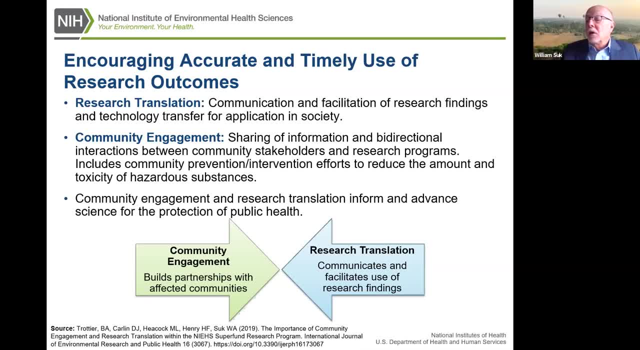 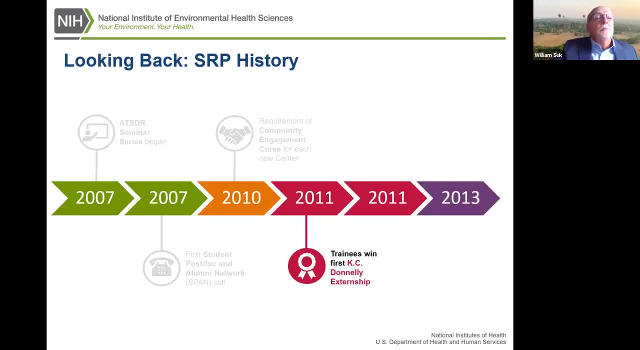 decisions about how to be able to decisions about how to be able to improve their health, Next, please. So the next one is the trail we started: the. So the next one is the trail we started: the Katy Donnelly externship Next, please. 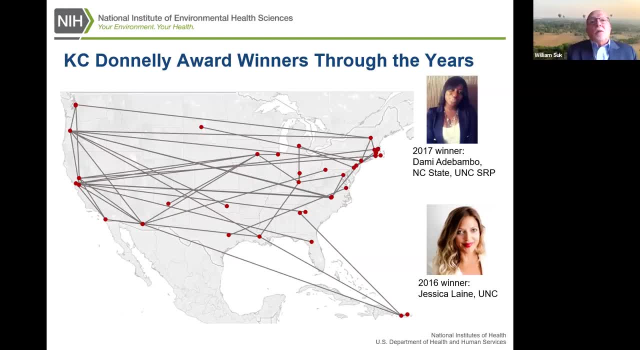 So this is. So this is. Katy Donnelly was a gentleman whose University of Texas- University of, I'm sorry, Texas A&M University, and he would, on his own, take students and move them into the field on a regular basis, and not only in this country, but also in other parts. 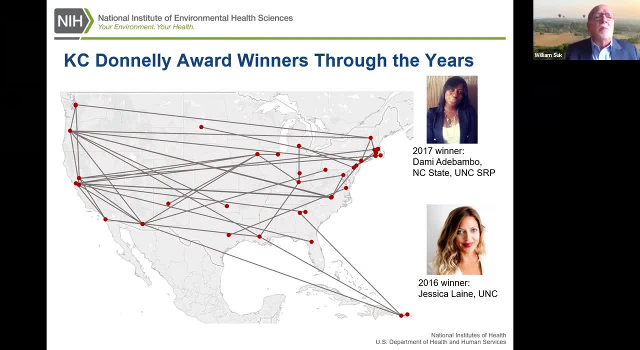 of the world. He would work closely with people in Azerbaijan, for example. and when Casey died, we decided to hold an award idea of bringing people back and forth between different programs to be able to learn different techniques. They can go to other SBIR institutions, They can go. 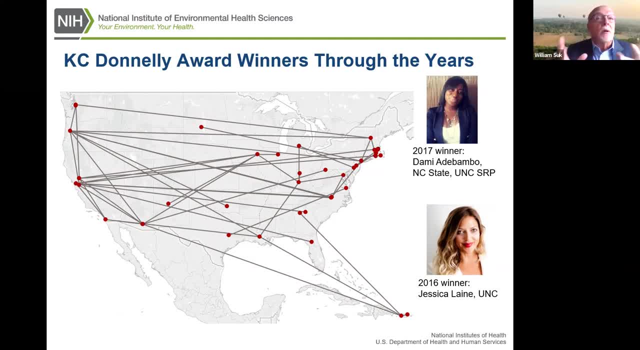 to government labs, They can go to state and local or tribal agencies. They can do anything they want, as long as it's within the context of that center's activity and it is going to help improve this individual's education. So in 2017, NC State and UNC winner was up there and in 2016,, Jess Lane next slide. 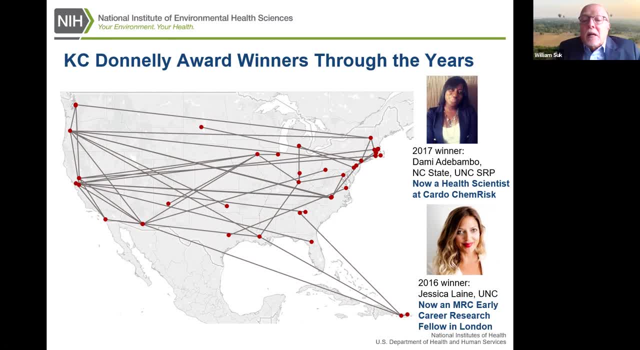 There we go. So now Dami is a health scientist at Cardio ChemRisk, which I believe is in um, I forget where it is exactly, but she worked with people at Columbia. okay, She worked with Mary Gamble at Columbia and um, no, she worked with 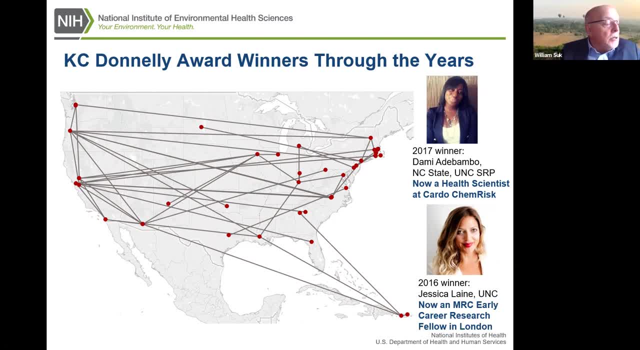 Anna Nava-Asian and Andrea Baccarelli at Columbia, and Jess Lane worked with Mary Gamble and she is now with the MRC Cancer Research Fellow in London. Next hit the button, please. and she is also a mom. 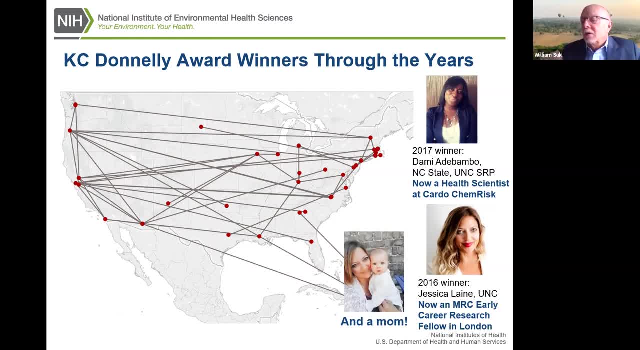 Um, I tried to. I keep in touch with her, um, because she's really very good at what she does and she's a nice person, and, um, uh, her daughter's name is Eleonora, which I think is a beautiful name. Next slide, please. 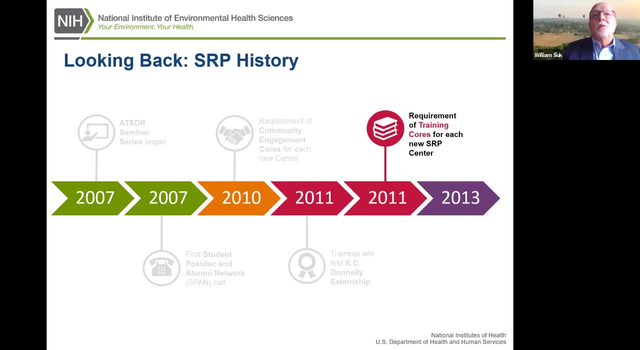 So, up until this point, training was not necessarily required as much as um running out of time, aren't I As much as um? anyway, next slide, please. But we feel that training is so important that it is now. 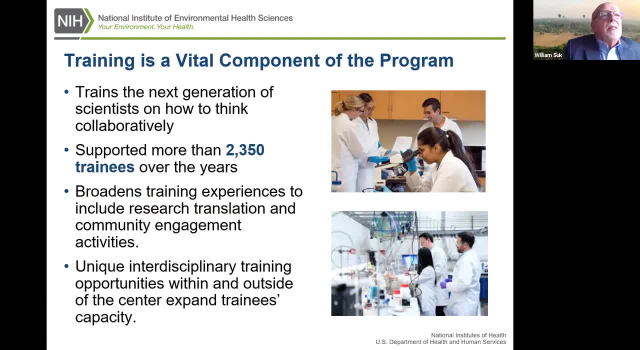 a required element within the program. Yes, it's easy to say we are training the next generation of scientists to think collaboratively. Yes, we are, but we're also training them in ways to think collaboratively- collaboratively with people who are not necessarily within their own. 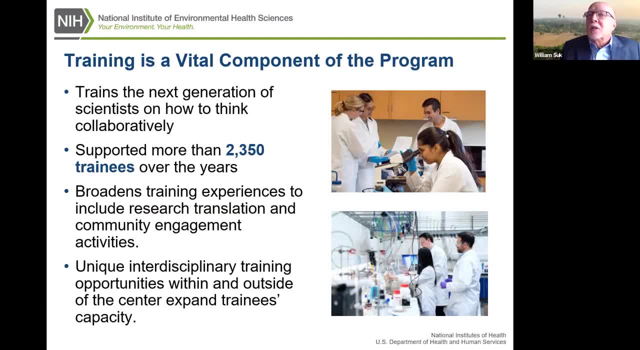 scientific discipline and that can also be a challenge for the future generations. So I think these sessions are very important and that can also be a challenge, but it can also be a real opportunity. So far, we've supported over 2,350 trainees over the years. 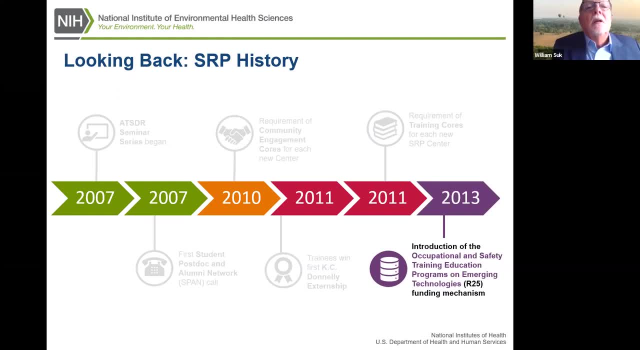 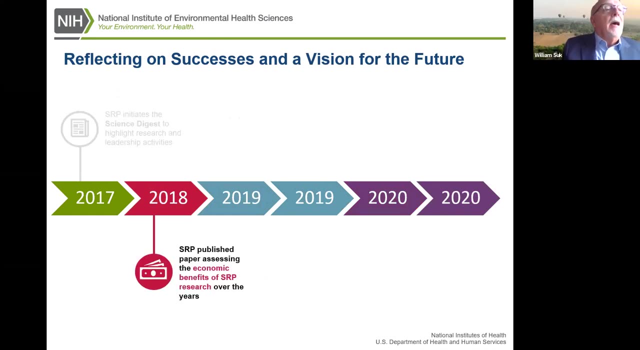 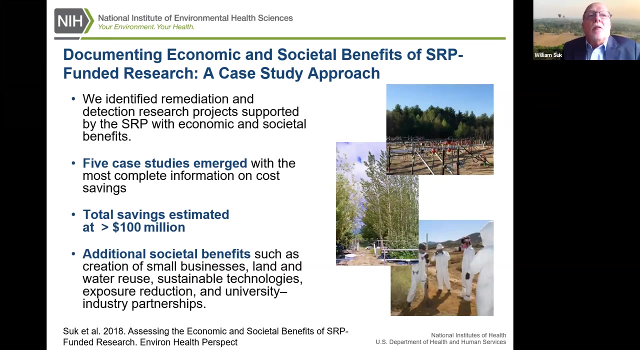 Next slide please. Recently, we've introduced an occupational training and educational program, an R25 program- Next slide please. And science digest: next slide please. And I mentioned that slide that moved before about how important economic benefits are- Next slide please. So a few years ago we actually documented the economic and societal benefits of our funded research. 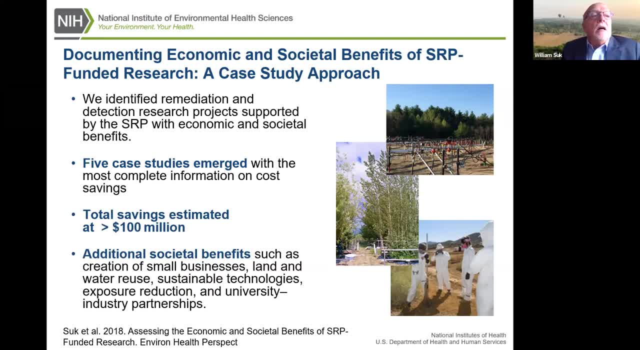 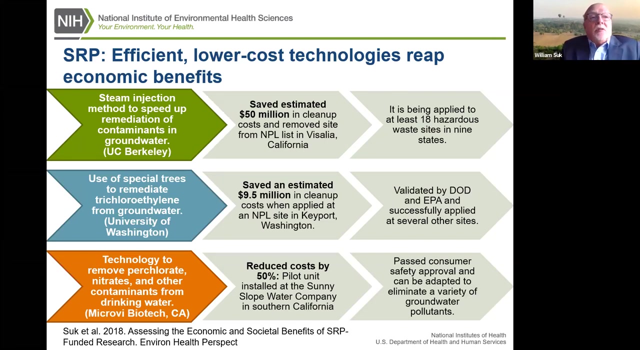 And we've demonstrated that what we did was we took the environmental sciences and engineering and did that first, And we estimated that we've saved over $100 million by developing sustainable technologies. Next slide, please. So these are some of the examples That we've cited. 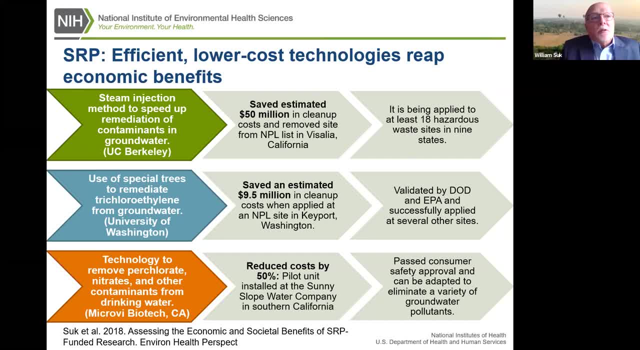 Steam injection method. that was done by Kent Udell at UC Berkeley and it's estimated to save us $50 million and it is being applied to at least 18 hazardous waste sites in nine states University of Washington. that's the work of Milt Gordon and he used poplar trees to actually 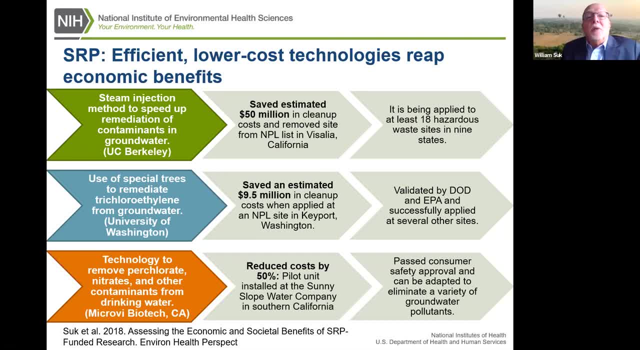 remediate trichloroethylene and that is being used and validated by DOD and EPA, and a company has developed a technology to remove perchlorate and has reduced the cost by 50%. My point here is that these are efficient, low cost technologies that reap economic benefit, that that are benefiting everyone. Next slide, please. 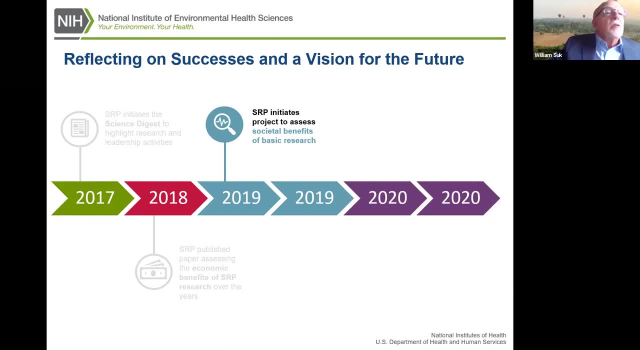 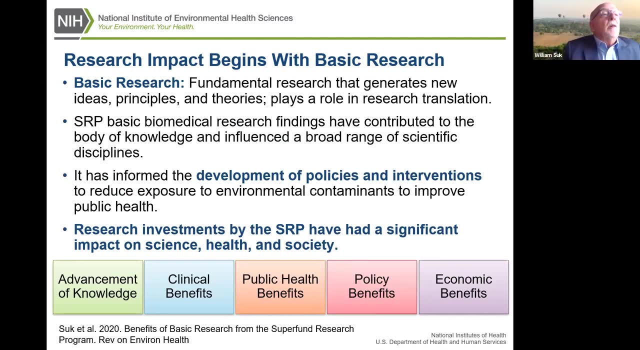 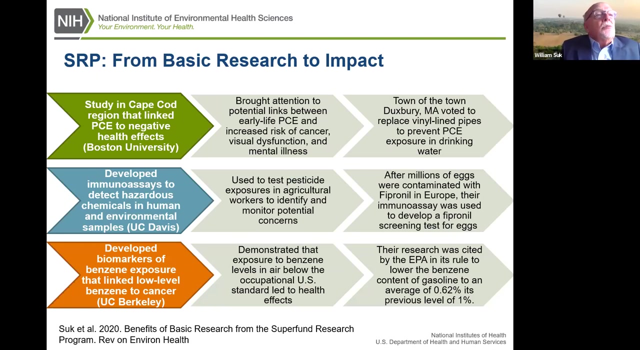 So we did the same thing with the basic fundamental research. Next, please, Where we look at the basic research in the biomedical research area primarily, That have contributed to body of knowledge and influence a broad range of scientific disciplines. Next, please. So these three studies that I'm citing here have had a significant impact on the environment. 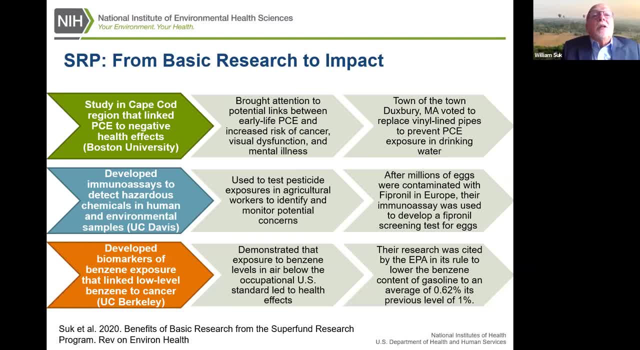 on the population in which they are working. The first one is Anne Ashingow. The second one, from UC Davis, is Bruce Hammack. The third one is Martin Smith's work demonstrating that exposure to benzene levels of air below the occupational standard led to health effects. 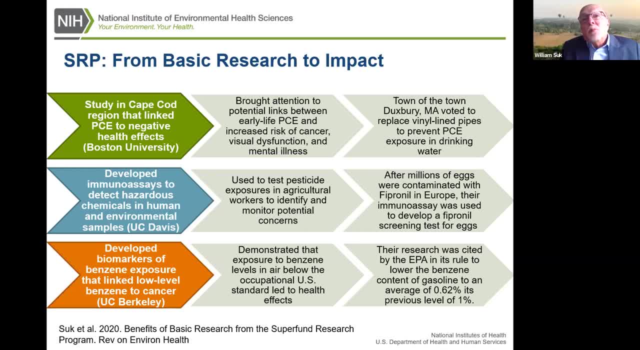 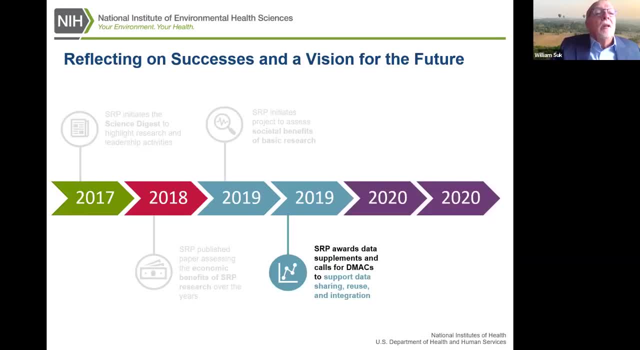 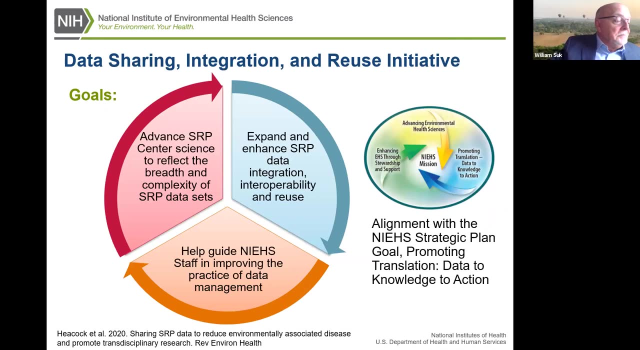 Okay, so they changed the rule. This has a significant impact on people's health and wellbeing. Thank you. Next slide, please. And then we get into next, please, the whole idea of DMACC and what we're doing. Last year, we actually put out an announcement. 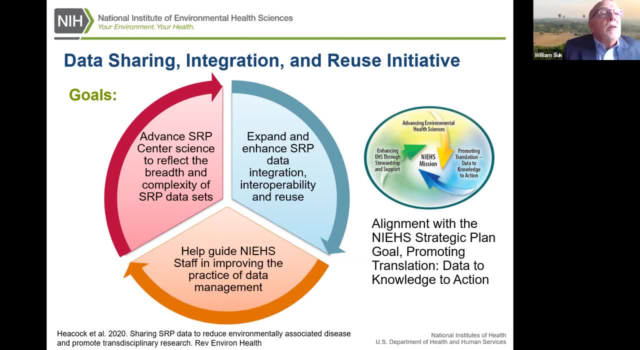 to allow people to advance scientific research. The point here is very simple: Data sharing, Integration and reuse is absolutely essential if we are going to address the problems that each of these that we're trying to face. The idea here is very simple, but it's not simple. 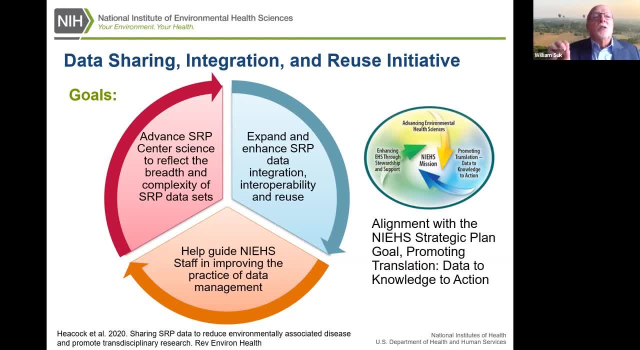 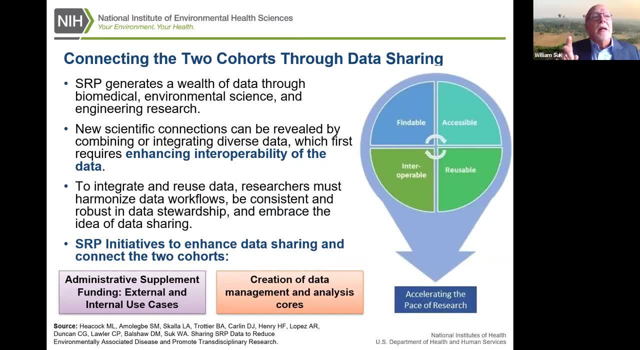 And that is, we're trying to develop the interoperability and reuse of the data within the program Next, please. So what I'm getting at is that we already have people. We already have people working together in different disciplines, and they're working together and the data is going into their own individual database, for example. 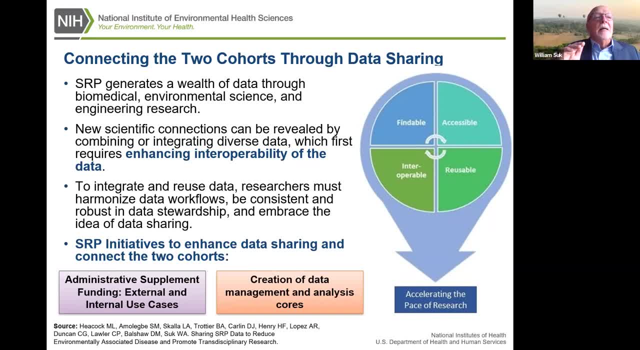 So the idea here is to be able to get data to be integrated and to enhance interoperability of the data. What I mean by that is that you need to have different databases talking to each other, because we need to address questions that are difficult to address and complex, and then, therefore, in order to do that, we need to be able to have different databases talking to each other. 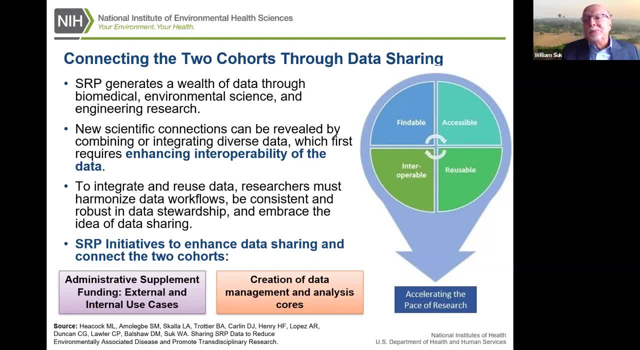 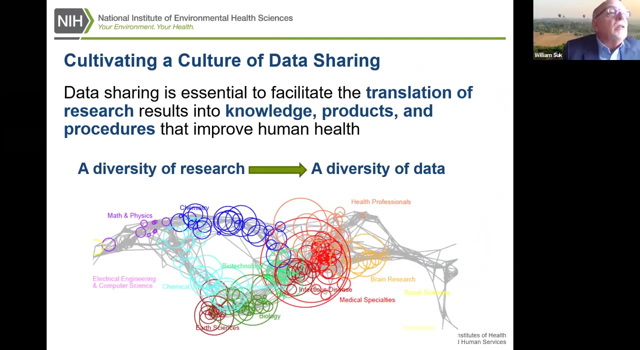 The idea is to answer questions that one, two, three, four disciplines can't answer on their own, but a variety of databases can answer these questions because of the interoperability of the data that we're trying to accomplish. Next slide: And this next slide kind of gives you an idea about the diversity of the research. 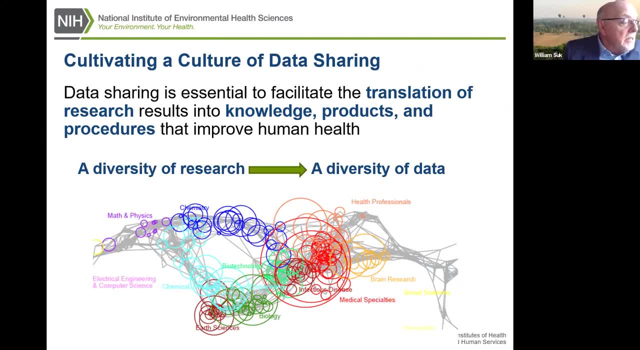 These are the actual. this is the actual data points that we have for the program. Again, this goes back to the map that I showed you earlier on, But the point here is: I don't know. So so, yeah, I do have some thoughts, But anyway, 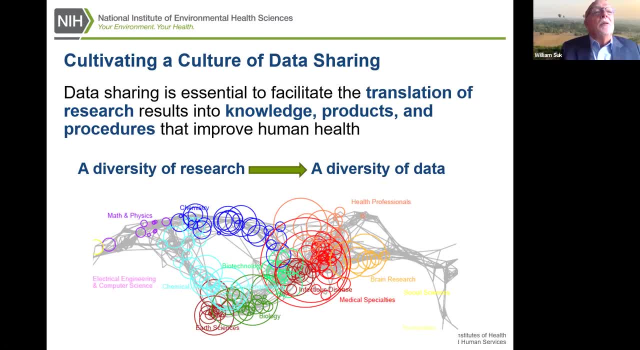 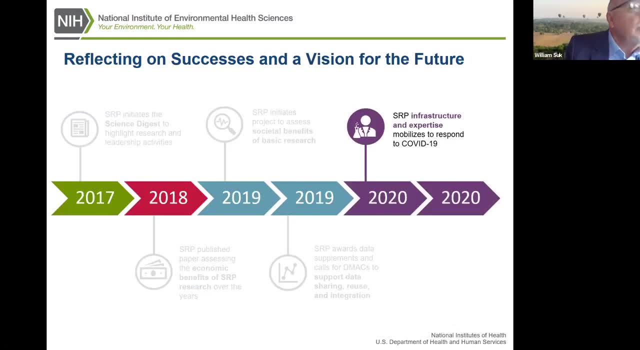 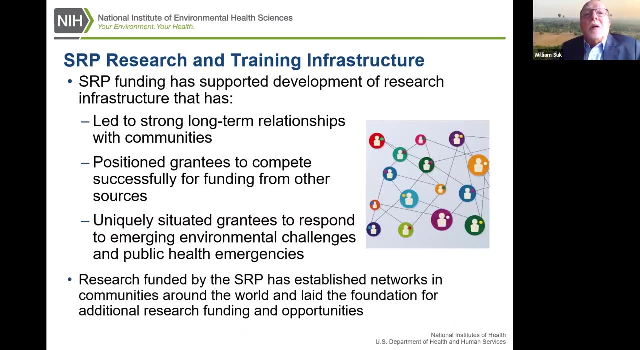 the whole idea here is to be able to develop, to be able to take advantage of the diversity of the data. Next, please, All right, next. So we have a situation and it kind of goes to what was just asked in the question as to the research and training. 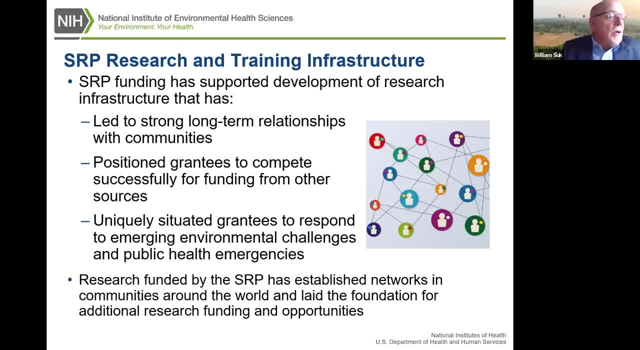 The Superfund Research Program has done a lot with regards to- yeah, with regards to- COVID-19.. It's been our research and our training infrastructure that has allowed organizations such as UNC to actually use the scientific background and infrastructure that they have in order to work more closely and develop tools that can help in this pandemic. 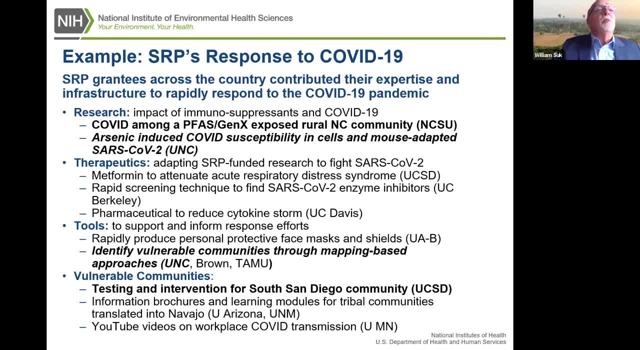 Next, please? These are just some examples. We have a whole part of our website that's dedicated to this And the research. we've done a lot of research on this. So at NC State they're looking at PFAS and Gen X exposed in rural population. 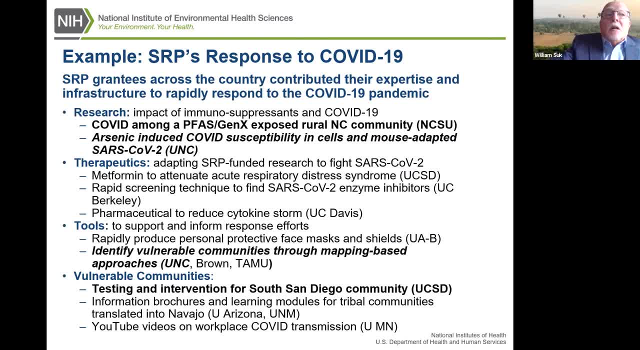 but they're looking at it within the context of COVID Here at UNC. they're at UNC arsenic-induced COVID susceptibility in cells and mouse adapted. And the other part of this is the one down below which says: identify vulnerable communities using GIS types of approaches. 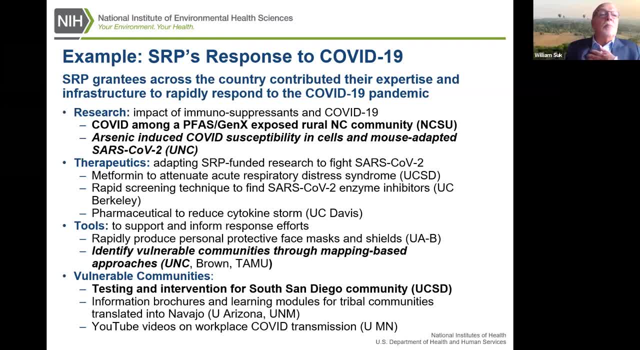 This is being done at UNC, Texas A&M and at Brown, But the whole idea is that you can't do this alone without having the research infrastructure to come to cast. at the moment it needs to, And I just highlighted the one on the bottom because at UC San Diego, 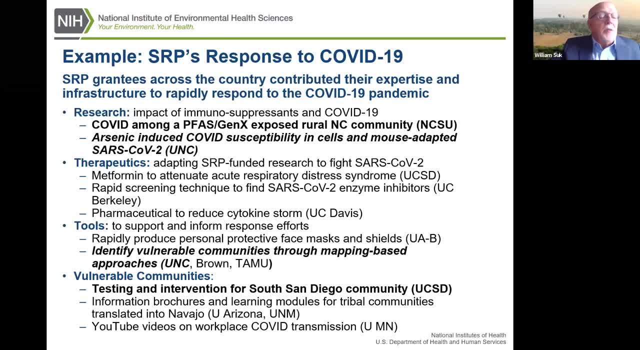 they're actually been supported by what's called RadX Up, which is an NIH initiative with regards to the response to HIV. So that's the response to NIH's response to COVID-19.. But again, they would not have been successful if, in their award, had they not had the research infrastructure necessary to accomplish what it is. 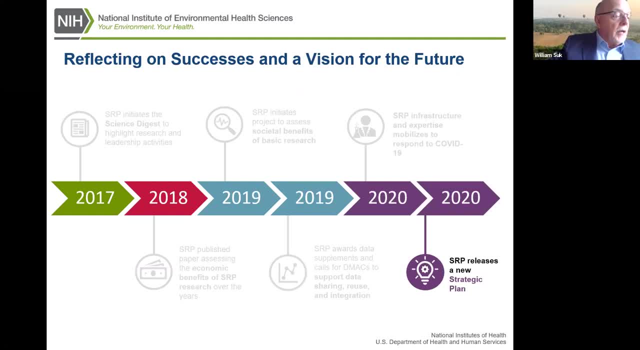 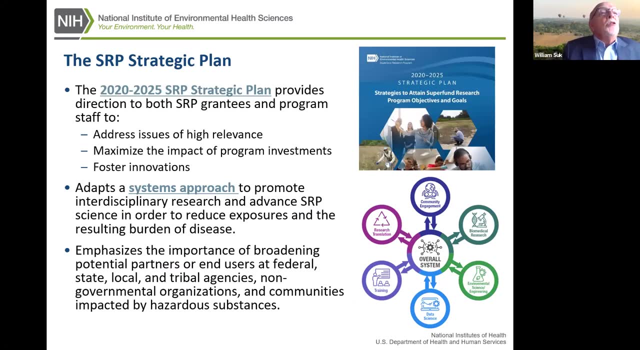 Next slide. So we've released a strategic plan. Next slide, please. I'm almost done, folks, Sorry. So the strategic plan provides for 20 to 25, 20% of what had been done in previous strategic plans and adheres to, links very closely or integrates very well with the NIEHS strategic plan. 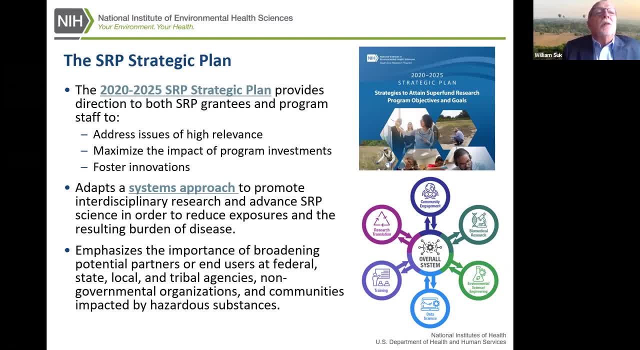 But we've also adapted a systems approach to promote interdisciplinary research. Again, this whole idea of being able to get people to work together across disciplines, across boundaries, and broadening the partners that we can work with- Okay, Not just EPA and ATSDR. 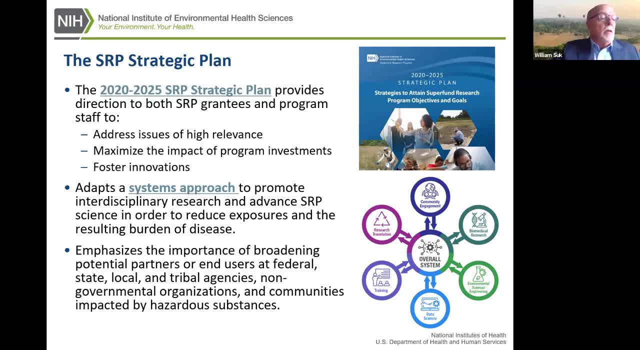 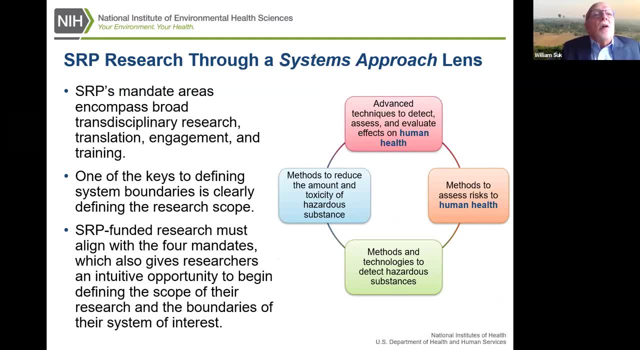 but also the National Science Foundation, NOAA, NASA, et cetera. Next, please, We still do this within the context of our four mandates, And that's important. The mandates encompass a broad approach to things. The key is to be able to address these things. 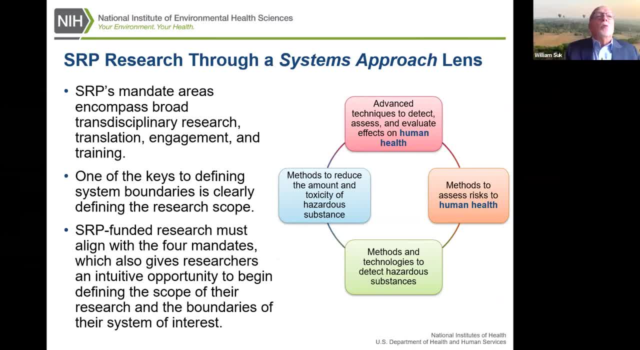 address these mandates using a more systems approach, lens in transdisciplinary, interdisciplinary research, taking full advantage of data integration and interoperability of data, and to be able to actually work together to address problems that can't be solved on their own. Next, please. 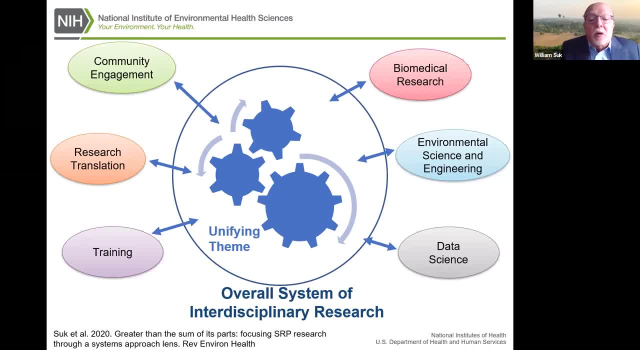 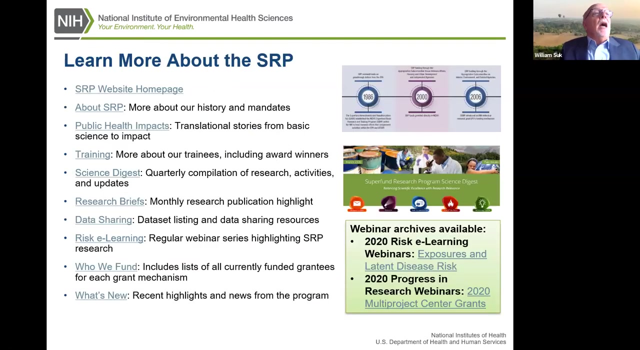 So this is the overall system Of interdisciplinary research, Again a unifying theme And bringing together these different components to actually make to address problems and to solve problems. Come up with solutions Next, please. So everything I've said you can find on this website. 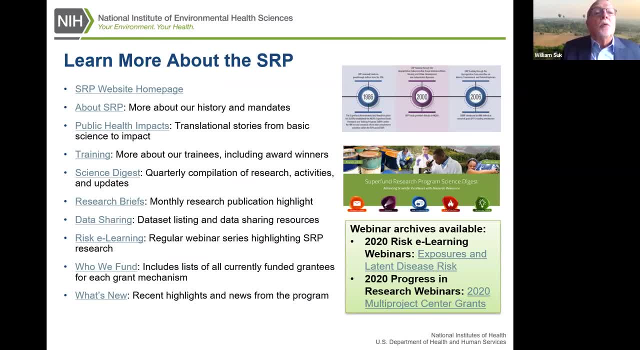 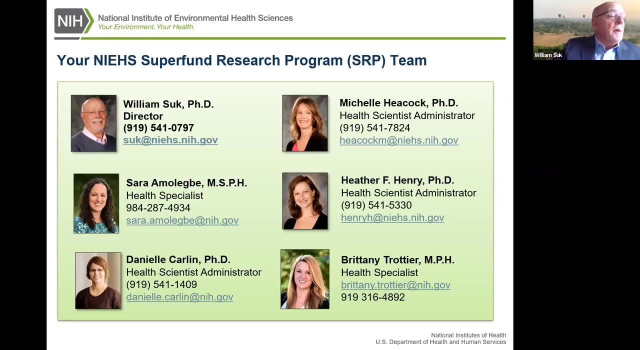 Okay, We will be doing, including. I mentioned that the webinars have been archived. Everything has been archived. The research briefs, everything is here, So you can learn more about the SRP. Next, please, And this is. 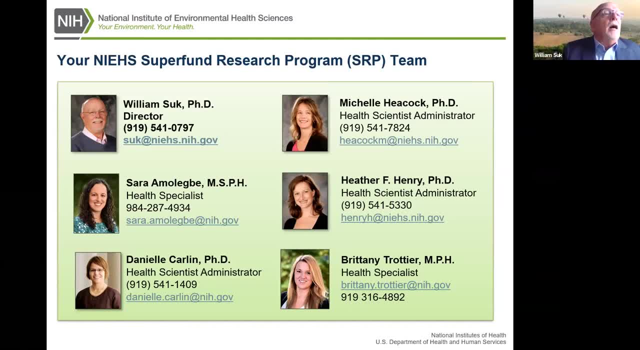 these are the people that do all the work. Okay, These are our email addresses. You have any questions? give us a holler. Seriously, they do all the work. And last slide, And the reason it's important to do this in a comp. 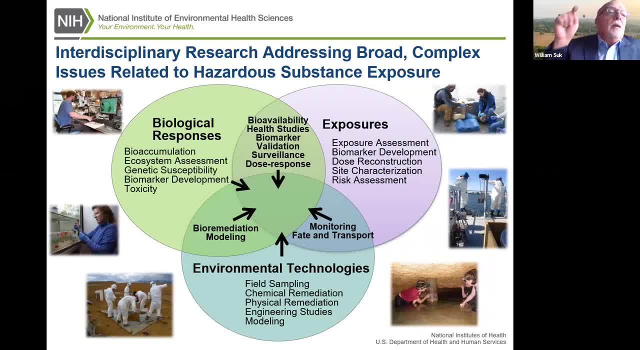 because this is a complex issue. These are all of the areas of research that we support And the focus, hit the button- Is to improve public health, And that's the bottom line. I'm sorry I went over, but I got excited about putting this together more than I did about 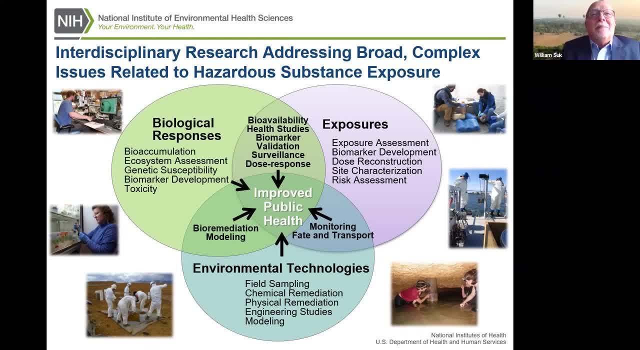 anything else recently. So so if you have any questions, I'm available. If you want to get up with me later on, I'm available, I'm always. I'm here, I'm not going anywhere. Thank you so much. 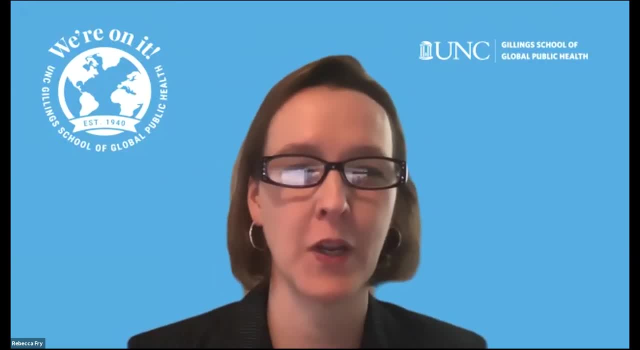 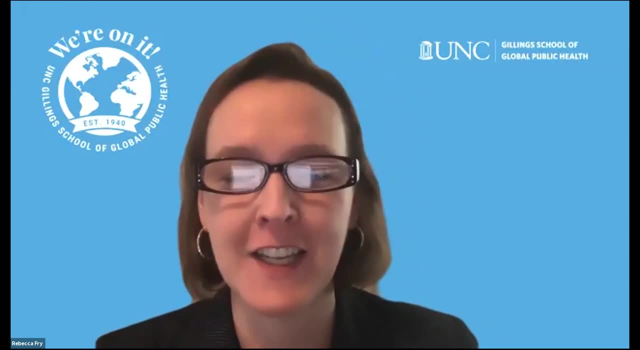 Bill, We have just a few quick questions from the audience. You had a great turnout and everyone is clapping for you, virtually Watching. this One is: do you have any advice for the next presidential administration regarding the what and how of environment and public health protection? 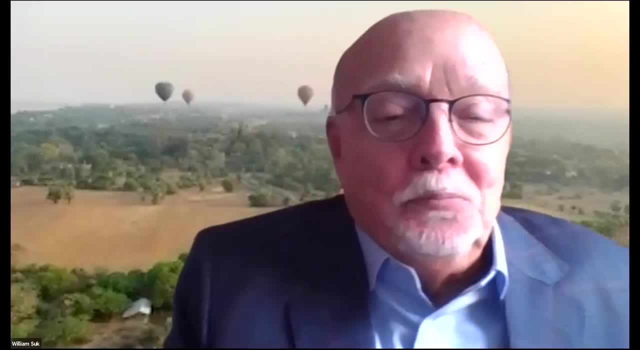 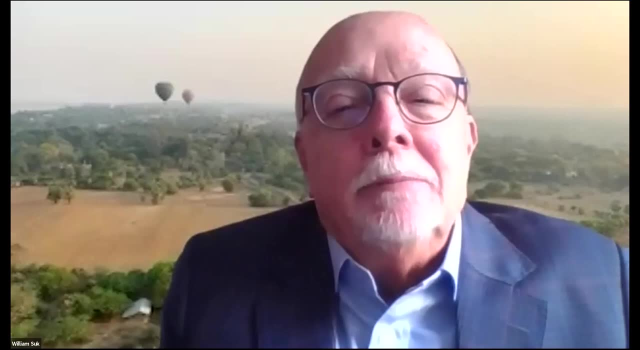 Yeah, Okay, Hmm, I'm not even sure I know where to start. Okay, I'm going to say this in two ways. One is that I think that The pandemic that we were experiencing has pointed up Many flaws in our public health. 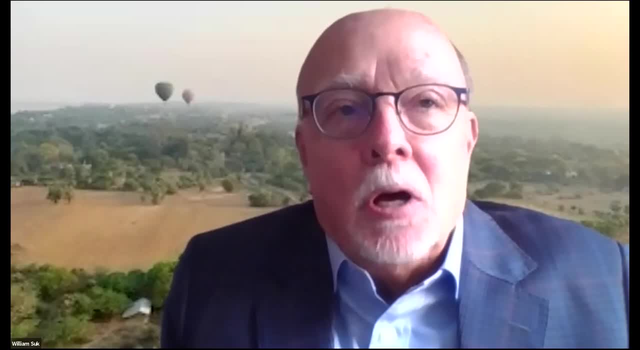 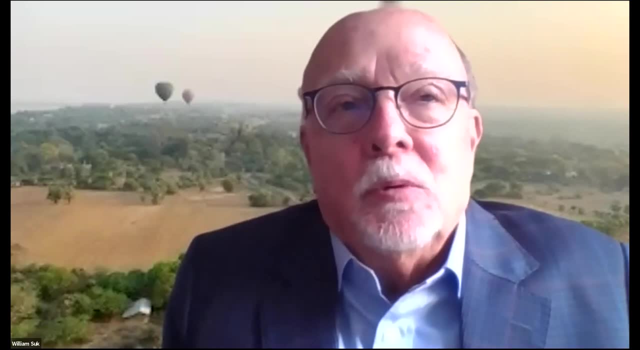 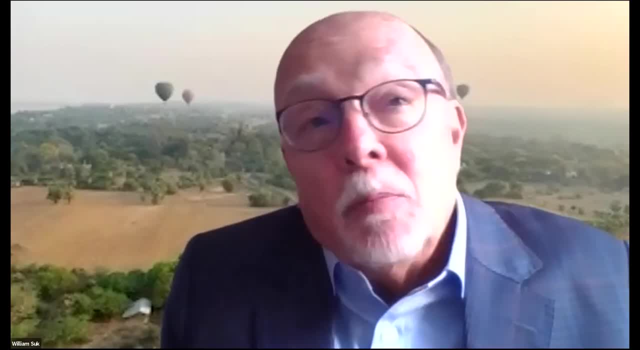 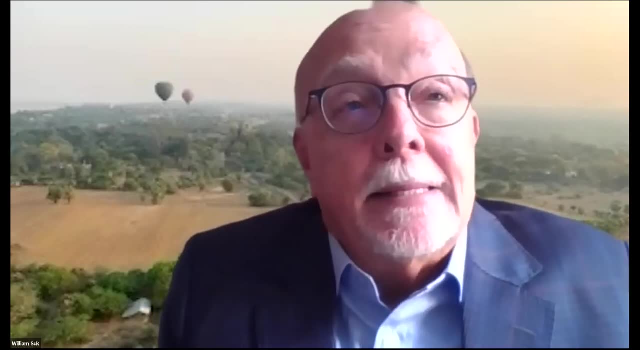 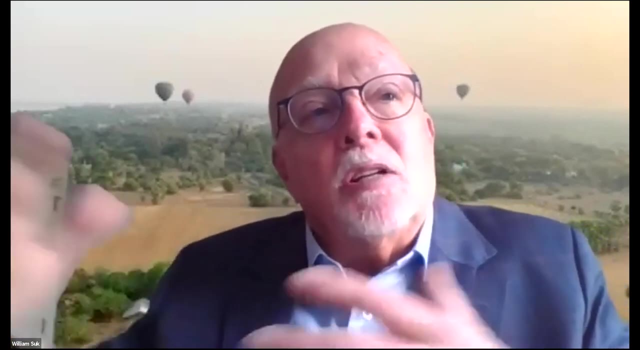 We have been working on a paper for a while. It's looking at, and there's been other papers that have come out that demonstrate that environmental exposures Set up As make worse. however you want to call it COVID and COVID infection, or the path of the pathogenesis of the